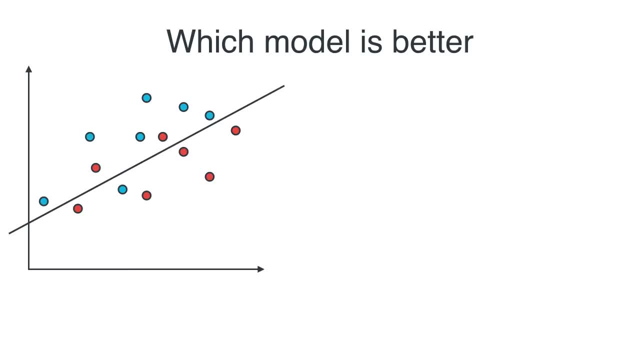 data. So our simplest model is this linear model, which is a line that cuts the data in two: blue and red. It makes some mistakes because there are some red points in the in the sort of blue area and some blue points in the red area, but in general it's a pretty good model. But 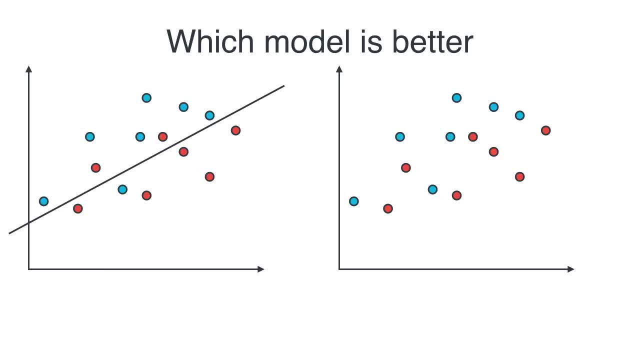 let's look at another model, a more complex one, So a higher degree polynomial, and this is how it goes: That one is seems to do much better with the points. It gets all the blue points on one side and all the red points on the other one. So here's a question: Which model is better between? 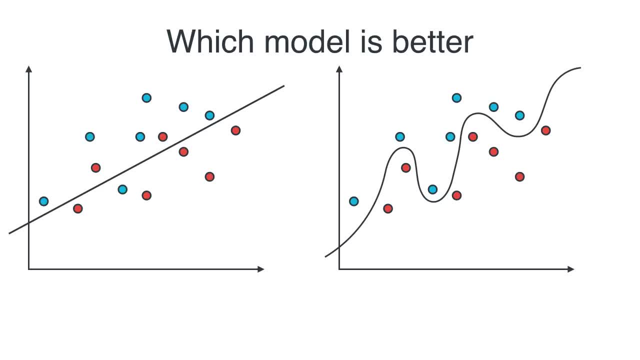 these two. I'll let you ponder on this one, That question, and let's see some methods to to find this out. So what we're gonna do is called testing. What we're gonna do is we're gonna not use every single one of our points for training. Instead, we're gonna split them. 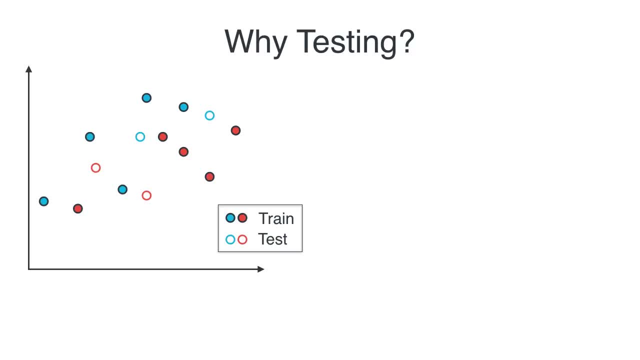 in two. We're gonna take a small portion of these points and call them testing. So here the the colored points are training. We used to train the algorithm, the model, and the points that are white inside they're for testing, So they're. 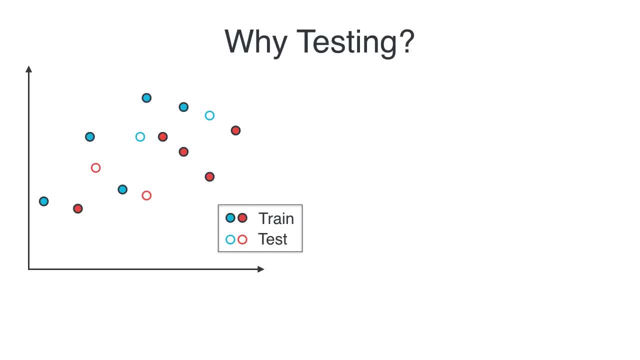 not, we don't see them. they're for testing. So they're not. we don't see them when we train the algorithm, but we we look at them later to test how the how the other model did. So here's again. our simple linear model Is this line: 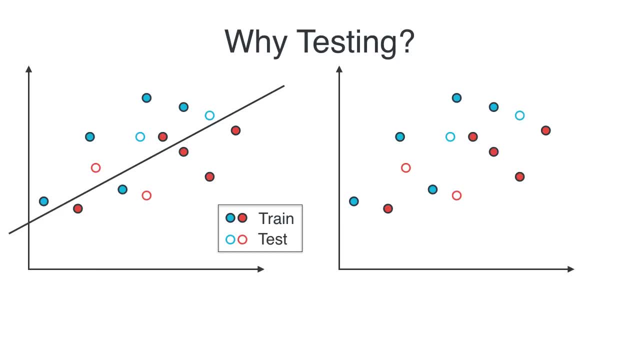 that splits the points into two. And now let's again look at the data split between training and testing and train a higher degree polynomial model here. So the model does this. It, as we said, it only looks at the training points and it does pretty well on the training points. 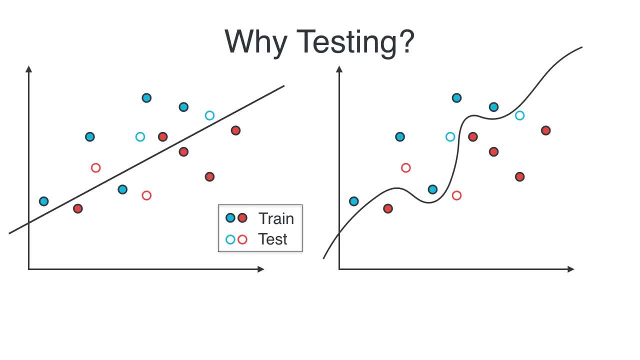 it, um, actually gets them all correct. and now, when we want to test the model, we just forget about the training set and we evaluate on the testing set. now, how does the model in the left do on the testing set? well, it only makes one mistake, which is this red point that is misclassified as blue. 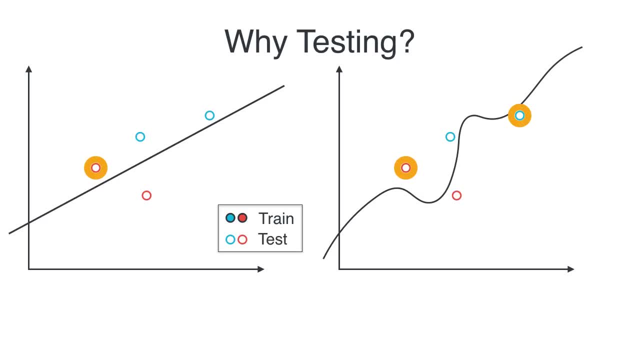 um, it's highlighted in yellow and the model on the right makes two mistakes, because it thinks of a red point as a yellow as a blue point and a blue point as a red point. so actually, when we look at the testing set, it turns out that the model in the left is better than the one on the 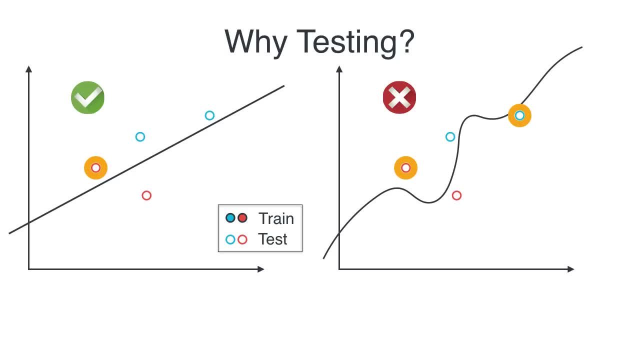 right, and the reason for this is that the one on the left just generalizes better, whereas the one on the right just kind of memorizes the data without really finding an interesting rule. so anyway, that's uh, that's testing in a nutshell. now there are some very important. 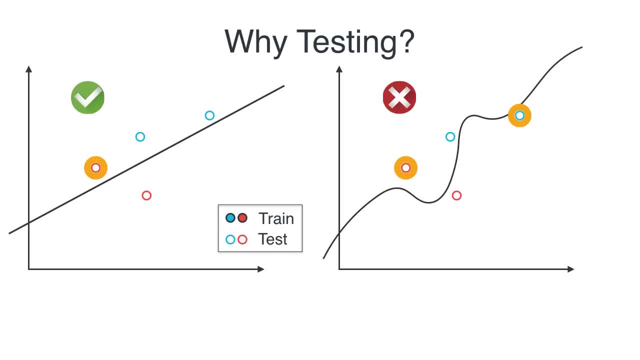 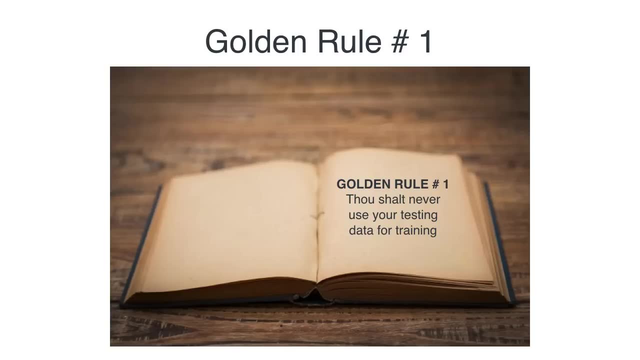 rules about testing. i call them the golden rules. so here it goes. golden rule number one: those shall never use your testing data for training. so when you take your testing data, you put it in the corner of the room and never look at it again until the very, very, very end. 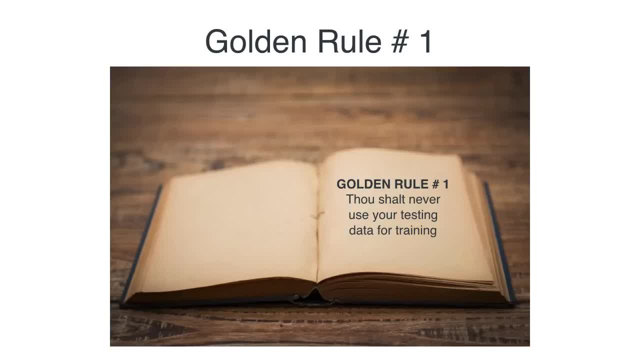 never use your testing data to to train your model or to make decisions about your model. uh, you'll see later how easy uh is it's to to mess this up accidentally, uh. golden rule number two says: friends, don't let friends use their testing data for training. so again, don't use your testing data for training. and golden rule number three says: 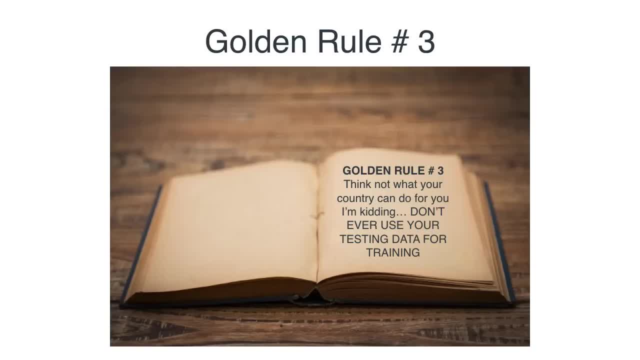 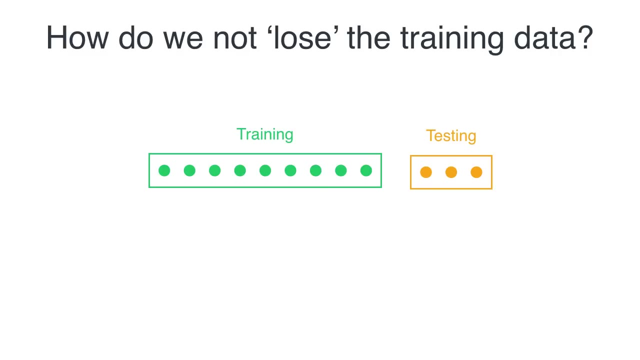 think not what your country can do for you. i'm kidding: don't ever use your testing data for training. so never, ever, ever, ever, ever use your testing data for training. but now this- this looks a little sad because it's it looks like we're taking some points and kind of throwing them away and not not using that. 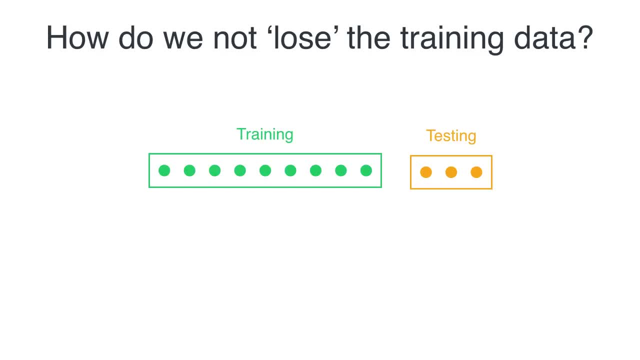 information very well. so there is, there's a way to kind of get around this. so let's look at our training points. are these green points and the testing points? there are these yellow points, and let's be a little redundant. so again, green training, yellow is testing. let's take our data and 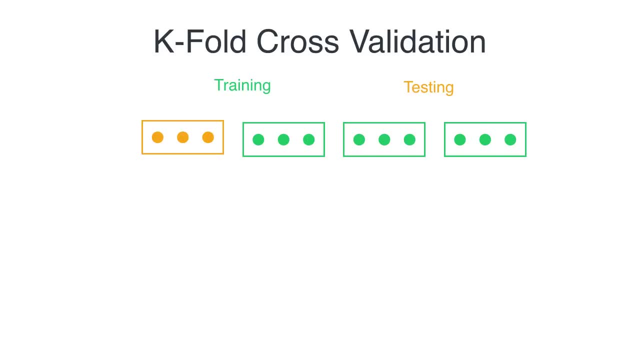 split it into k equal sets. uh. here k is four. so we take our data and split it into four sets and we use one of the sets as the yellow one for testing and the other three for training. and then we train a model, again using the second little little uh set for testing and the others for training. and then we do this again. 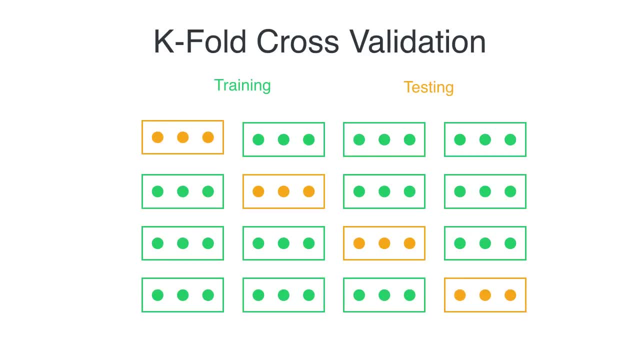 and again, and then at the end we average our results. so we basically each each portion of data is used for for training and for testing, and that actually works pretty well. normally, you would want to to randomize the points, so not just to randomize the points, but to randomize the points, and then we 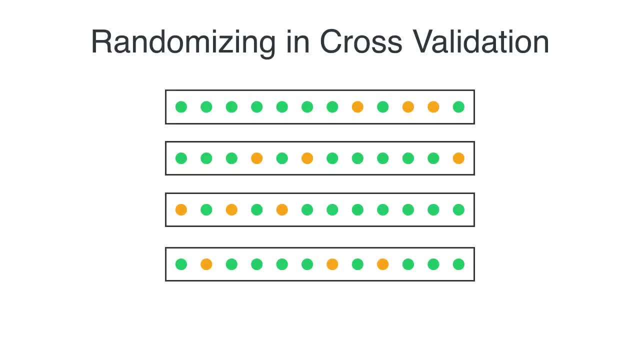 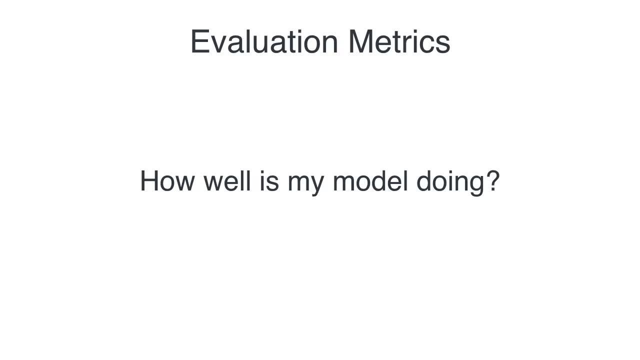 not not take the first uh, first k and then the second. you actually want to do this randomly, but if you see here every, every point is used for for training three times and testing another time anyway. so that's it for our testing sets. now we still have the question. 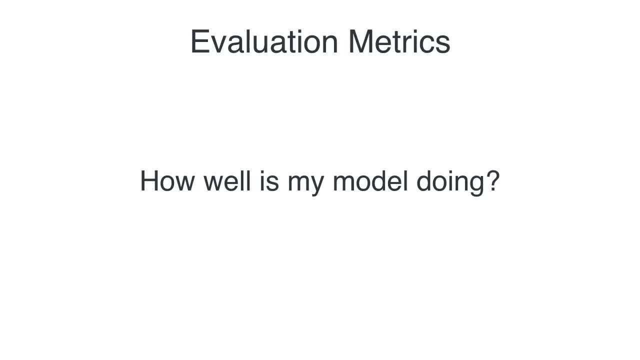 how well is the model doing? so let's look at some metrics that will tell us how our models are doing, and this can be a tricky question. let's think about it. what is a way to tell if a model is doing well? so first thing at the top of my head would be saying: well, if a model is correct most of the time. 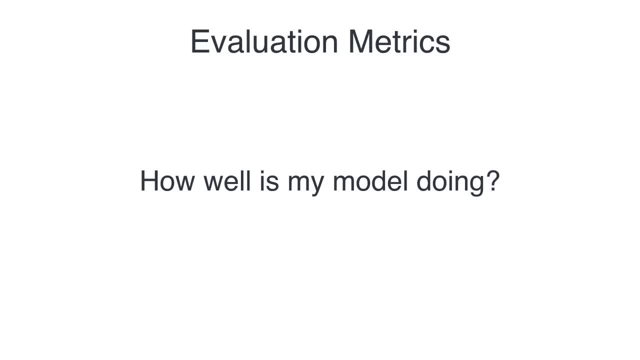 then that model must be pretty good, but this can- this can be tricky. let's look at an example. the example is called credit card fraud. so we have a bunch of data in the form of credit card transactions, and some of them are good, like the ones in the left. 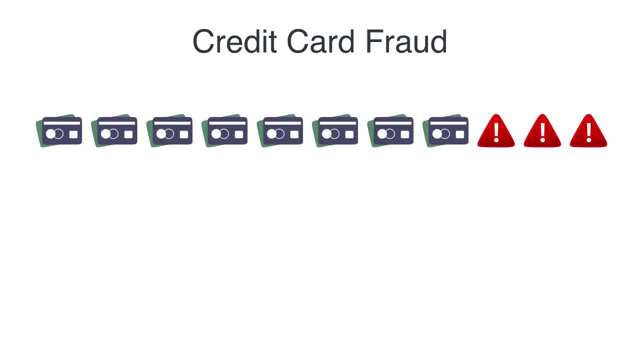 and some of them are fraudulent, like the ones in the right. uh, let's look at numbers. so there are 284.336 hundred and thirty five good transactions and 472 fraudulent transactions. is actually real data. so let's, let's think of a model and let's. 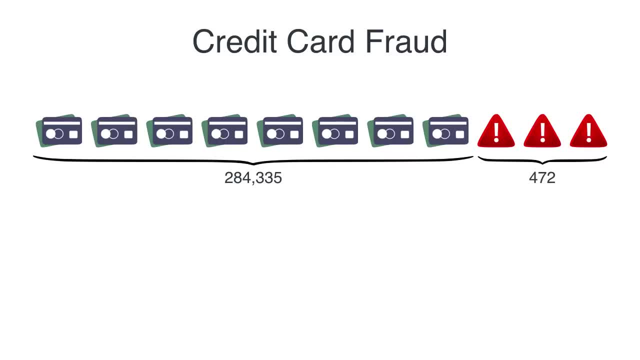 try to come up with a model that's really good, so a model that is correct most of the time. can you help me think of a model that is correct over 99% of the time? so here's a model that's correct over 99% of the time. the model: 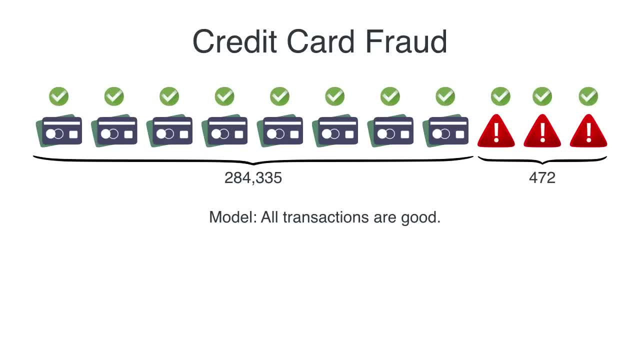 that says that all the transactions are good. so how many times are we correct? well, we're correct 284 thousand three hundred thirty five times out of two hundred eighty four thousand eight hundred and seven times, and that's ninety nine point eighty three percent. so this model must be pretty good, right? well not. 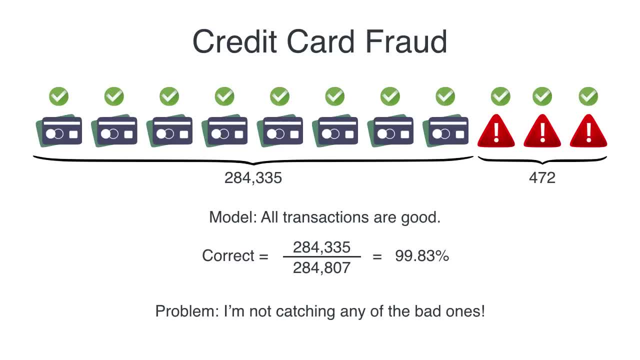 really, I'm not catching any of the bad ones, and the point of the model is to catch the fraudulent transactions. so let's look at another model. what about can we get a model that catches all the bad transactions? can we think of one? well, here's one. I'm gonna call all transactions fraudulent, so that's great. 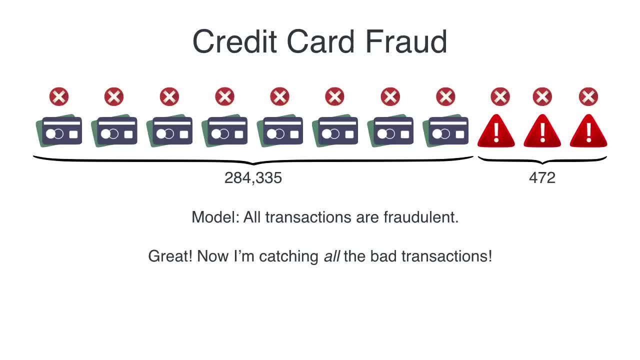 right now I'm catching all the bad transactions. is that a good model? well, now it's a terrible model, because I'm also accidentally catching all the good ones. so it's tricky to to try to think of how many times I'm correct and how many times I'm wrong. so let's go to another. 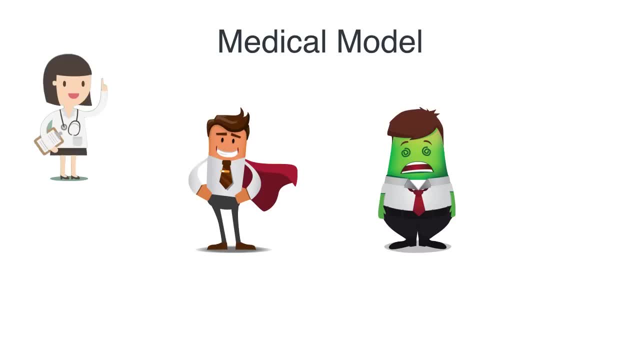 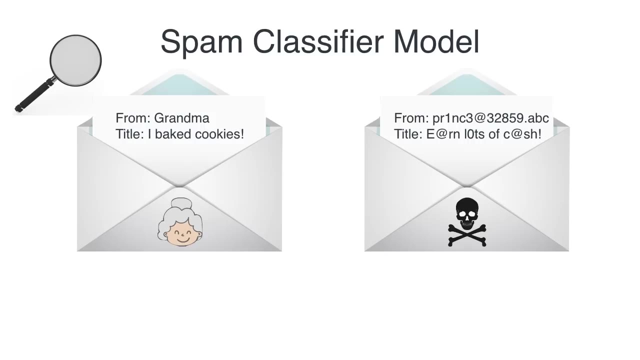 two examples that will illustrate this. we have a medical model, so the medical model is basically a doctor that tells you if you're healthy or if you're sick. that's our first model, and our second model is going to be the spam classifier model. so the spam classifier model looks at emails. for example, on the left we 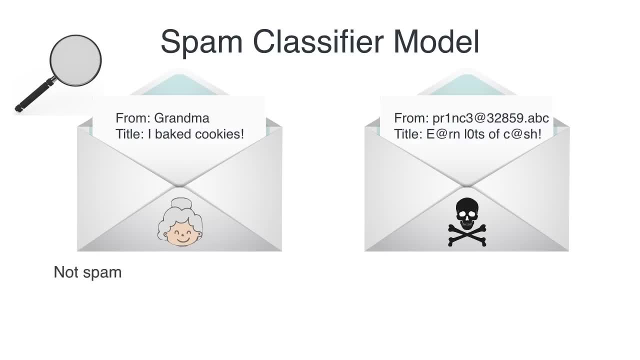 have an email from, from grandma saying I baked cookies. that's not spam, obviously. and then from the right we have an email that says: earn lots of cash from a weird address and it looks very sketchy, so that's gonna be a spam model. and so this, this, this is our second model. 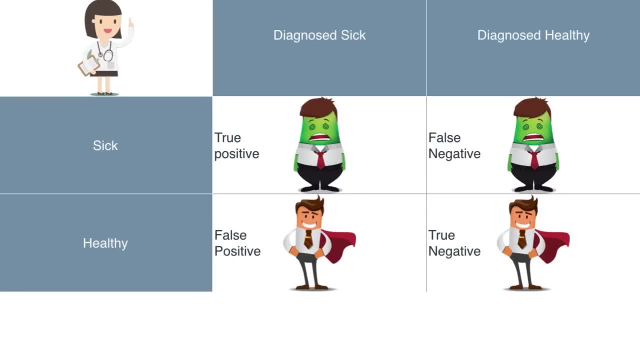 so let's look at what is called a. it's called a confusion matrix. this is a table where four things can happen. right, the rows say: are you sick or are you healthy? and the columns say: are you diagnosed a sick or are you diagnosed as healthy? and so, if you are sick, you're healthy. and the columns say: are you diagnosed as sick or are you diagnosed as healthy? and so, if you are, 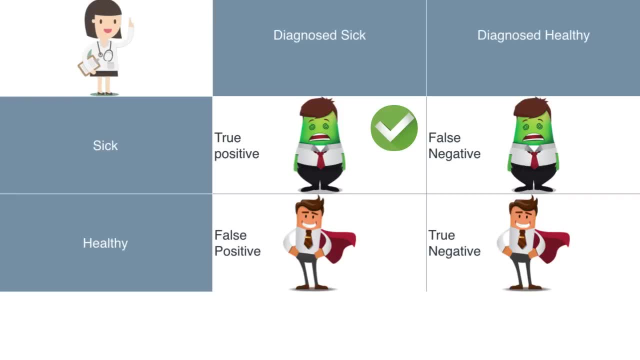 on this box, it means you are sick and you're diagnosed as sick, so the model did well. it's called a true positive. if you are on this box, you, the model was also good because you're healthy and you were diagnosed as healthy. if you're here, 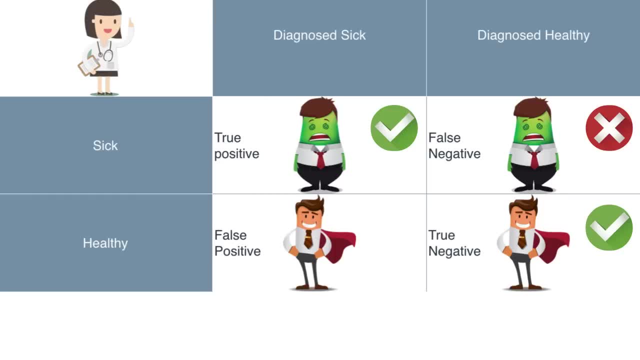 you're called a false negative. that means you are sick but you're diagnosed as healthy. and if you're here, you're called a false positive means you're healthy and diagnosed as sick. so those are our names. we're gonna use a lot true positive, false negative, false positive. 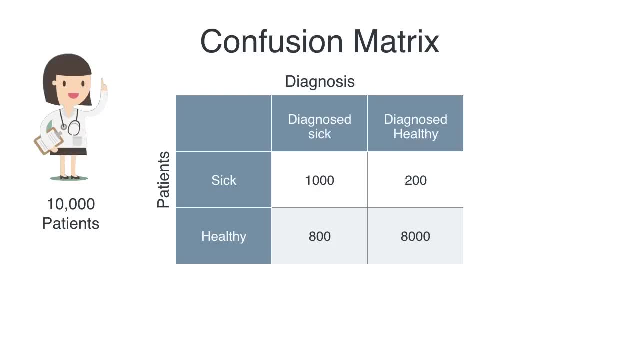 and true, negative and the confusion matrix given given some data like, for example, ten thousand patients. we're gonna look at how this model is doing so. there are a thousand two positives- sick patients that are correctly diagnosed as sick. there are eight, two hundred false negatives, which are the sick patients. 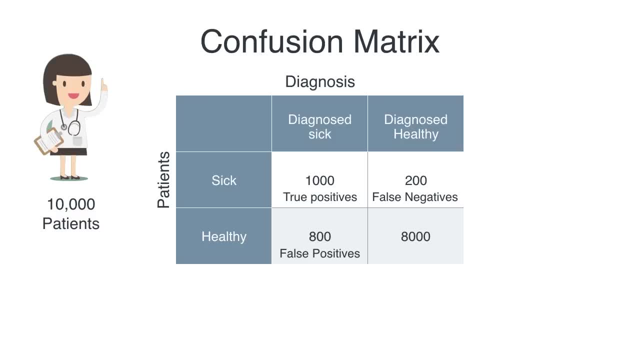 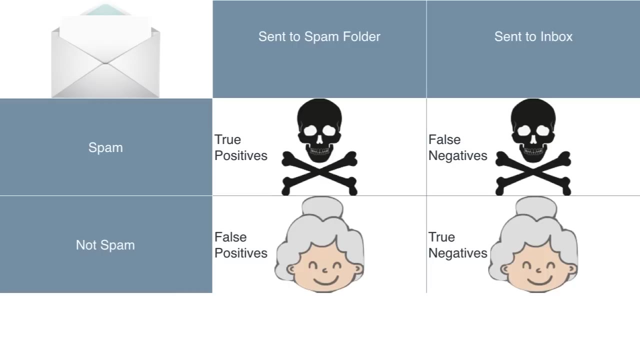 that I diagnosed healthy. there are eight hundred false positives, which are healthy patients diagnosed as sick, and eight thousand true negatives, so healthy patients diagnosed as healthy. okay, that's a confusion matrix. now let's look at our second model. so we have on the rows, we have spam and not spam. 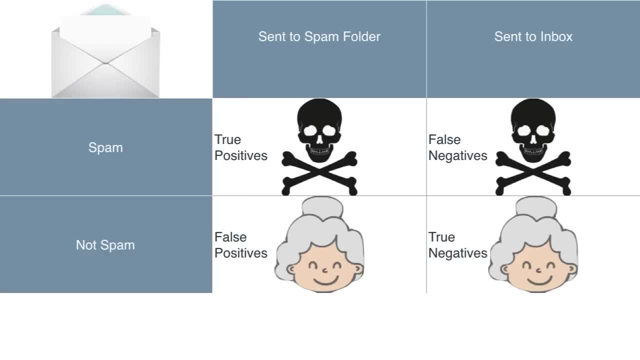 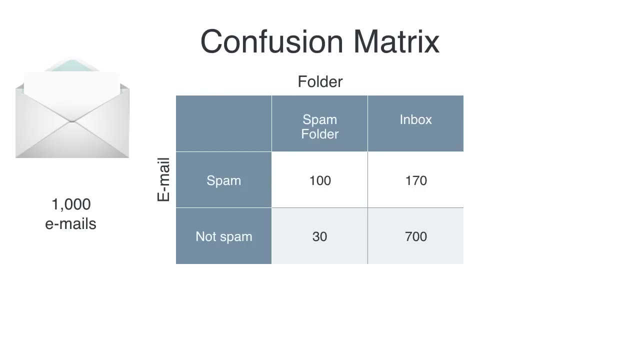 and on the columns, we have our sent to spam folder or sent to inbox, because we're going to take the messages that are not spam. we send to inbox. so we have our true positives, our false negatives, our false positives and our true negatives, and now we look at a thousand emails. that's our data. 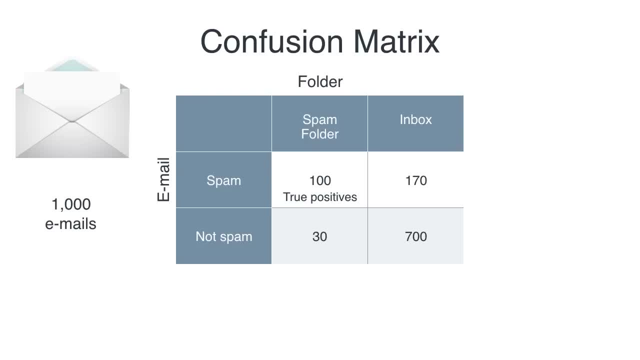 and we have that. a hundred of the spam ones are correctly sent to the spam folder as true positives. 170 of the spam ones are accidentally sent to inbox- that's false negatives. 30 of the not spam were accidentally sent to your spam folder, which is false positives, and 700 of the 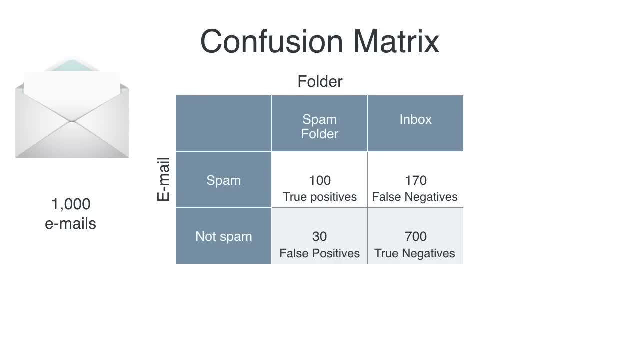 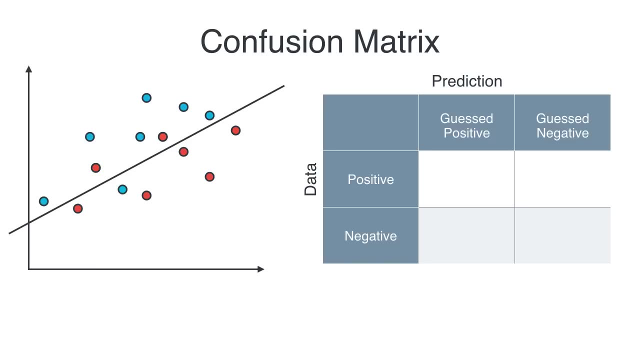 not spam, were sent to the inbox. so let's look at a a more graphical example. more graphical example is that the model from the beginning says blue is positive and red is negative. so maybe you can help me out filling this, this table. how many true past positives are there? I'll give you a minute. feel free to pause the video if 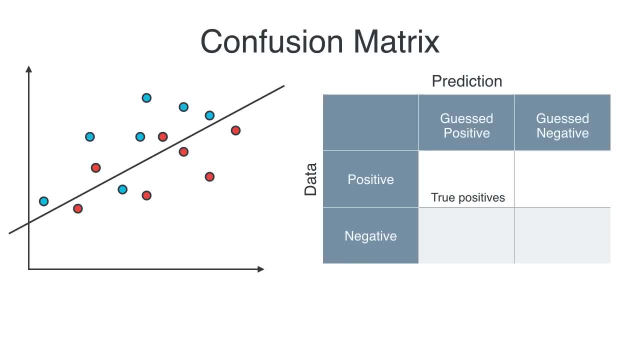 you want to think about it. so the true positives are the points that are already positive and guessed positive, so this one's right. so that means there's six of them. how many, uh, true negatives do we have? well, we have five points that are negative and also diagnosed as: 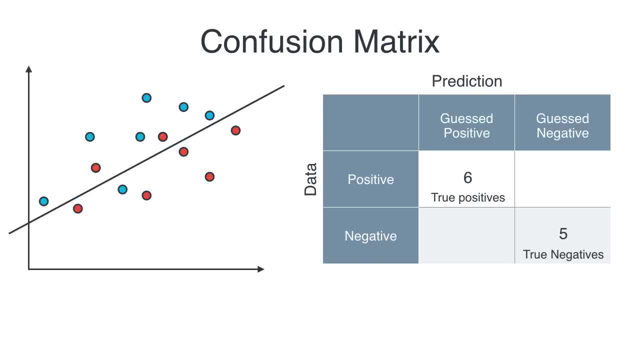 negative, so that's five. uh, what about false positives? well, these are the points that are negative, so they're red, but the the model thought they were positive. so it's these two over here. and finally, the false negatives are the ones that are positive but the model thought were negative. 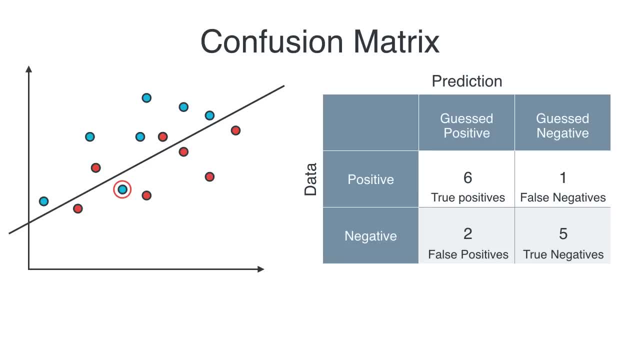 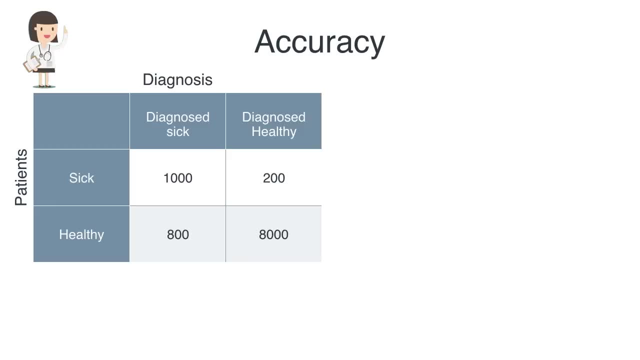 so it's this one over here, so one. so that's our confusion matrix for the linear model we saw at the beginning. so let's look at the first of our metrics. the metric is called accuracy, and accuracy is the answer to the following question: out of all the patients, how many did we classify correctly? so? 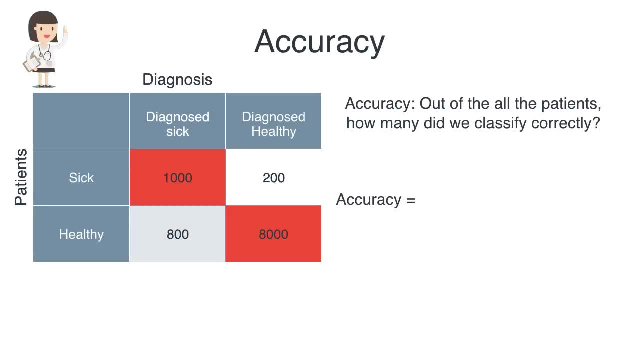 here the accuracy is the number that we classify correctly, which is the ones on these two boxes: ten plus eight thousand, so nine thousand divided by the total number, which is the number that we classified, which is ten thousand, so it's a ninety percent. the accuracy of the email model is out of. 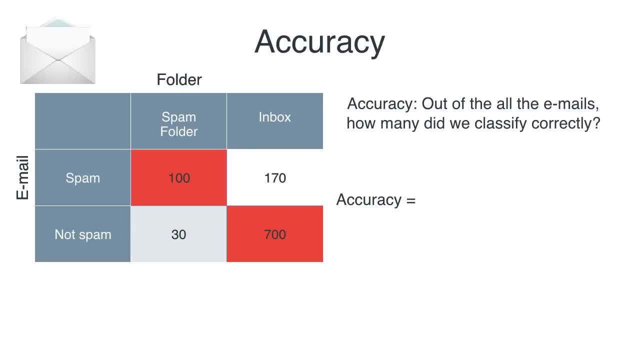 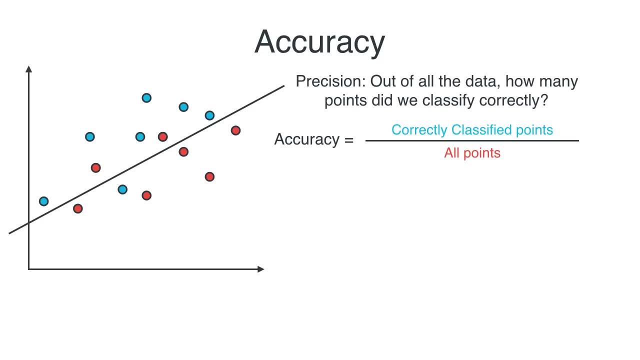 all the emails, how many do we classify correctly? so it's the ones in these boxes, which is a hundred plus seven hundred, divided by a thousand, which is the total number of emails. so it's eighty percent. and finally, in our linear model, again the accuracy is the number of correctly classified. 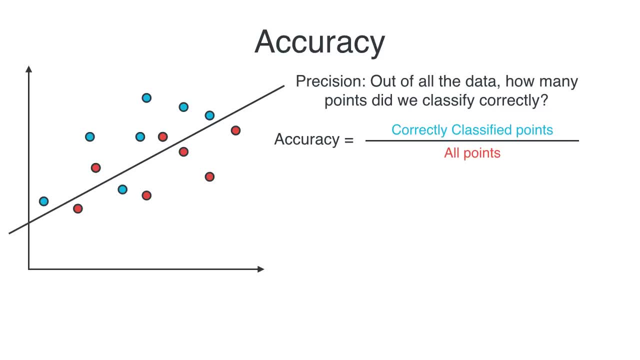 points divided by all points. so how many points are correctly classified? well, the ones that are positive and the model classified as positive, plus the ones that are negative and the model correctly classified as negative. that's these 11 points divided by the total, which is 14. so 11 divided by 14, that's 78.57 percent. but now, as we saw in the credit card model, 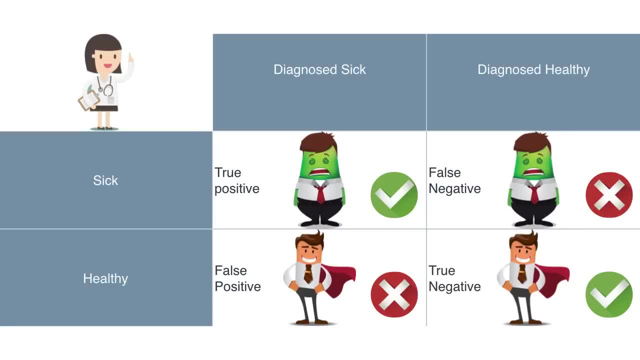 accuracy is not the best metric. so let's actually study the model a little more to see what metrics to use. so let's look at the credit card model and see what metrics to use. so let's look at the credit card model. so let's look at only the mistakes. let's forget about the cases when you diagnose a sick person. 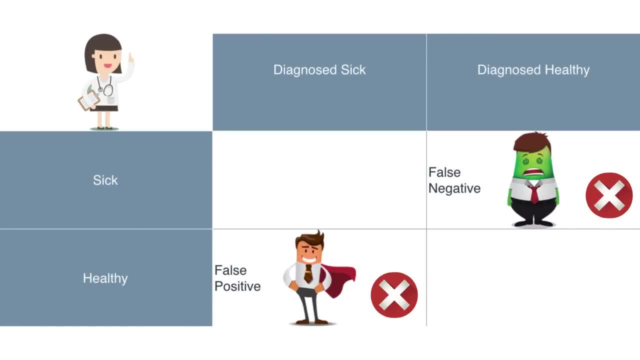 as sick and a healthy person is healthy. so we have two things that can happen, two mistakes we can make. we can diagnose a sick person as healthy, in which case we get a false negative, or we can diagnose a healthy person is sick, in which case we we get a false positive. so which one of these is worse? 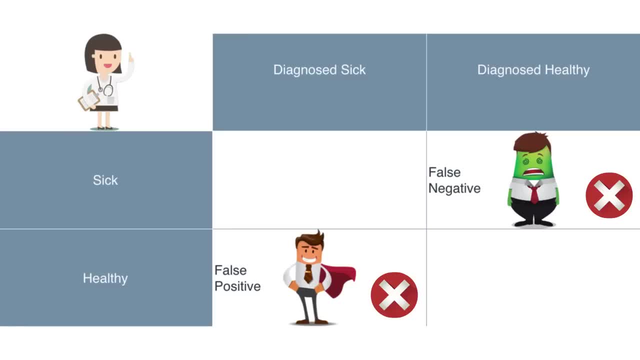 i'll let you think about it for a minute. so the the problem, the false positive, would be, uh, if we take a healthy person, diagnose them as sick and then we send them to do more tests, so that's kind of annoying. but the false negative means there's a sick person and we're sending 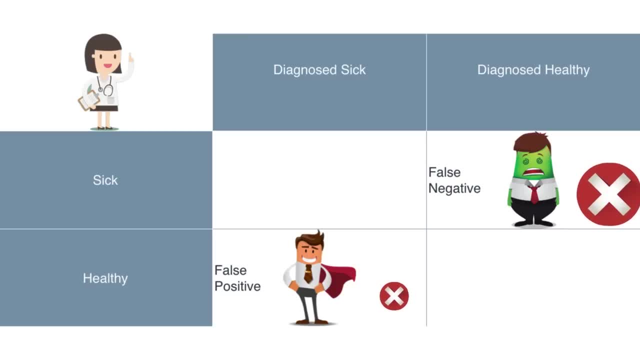 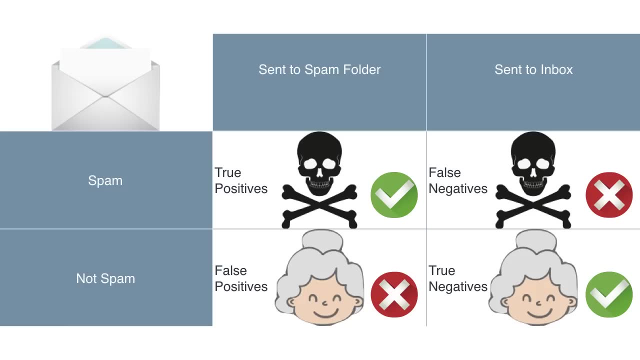 them home with no treatment, so that's much worse. so in this case, a false negative is a lot worse than a false positive. and now let's look at the spam detector model. so again, let's forget the times when the model got it right and focus on the mistakes. 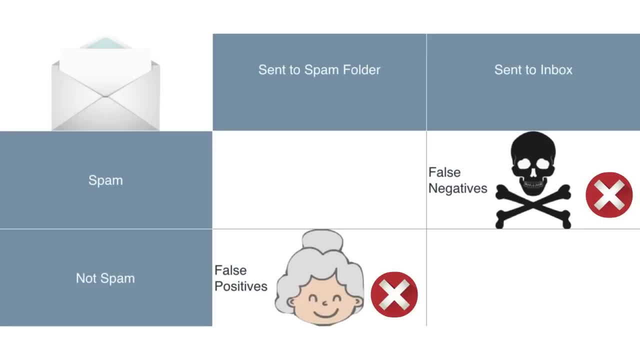 the two possible mistakes are a false negative, which is taking a spam message and accidentally sending it to your inbox, and a false positive, which is when an email from your grandma comes in and the model accidentally sends it to a spam folder. so let's, let's think about it again. that take a few seconds to. 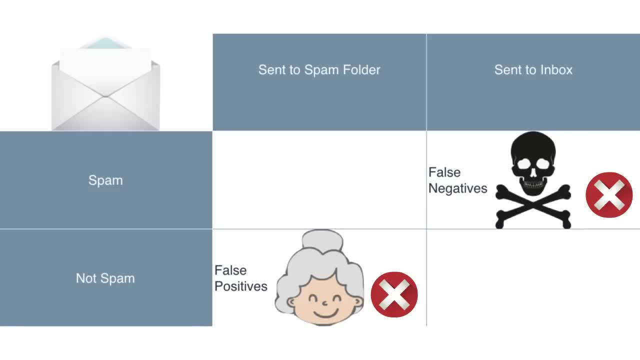 think about it, which one of these two mistakes is worse? so if you said false positive, you're correct, right, because the false negative is so it's kind of annoying, but it's okay. just means you've gotten a spam email sent to your inbox and you had to delete it manually, whereas the false positive that that'd. 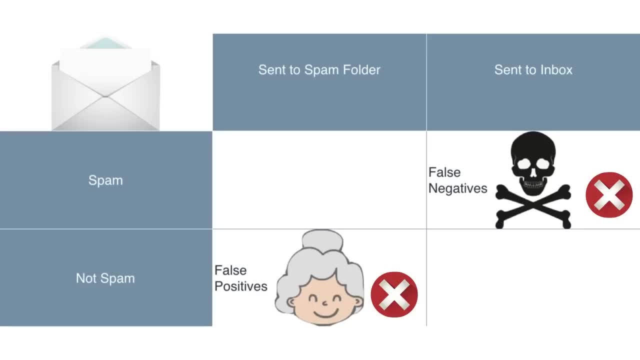 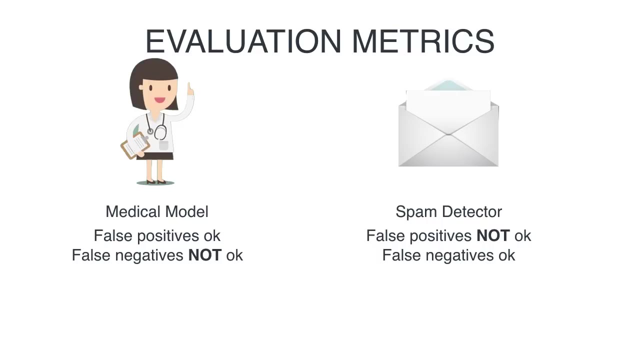 be terrible. the poor of the poor grandma, she, she learned to type an email only so she can send you an email to let you know that she baked cookies and you go and delete it. so in this case, false positives is much, much worse than false negatives and in that way, the medical 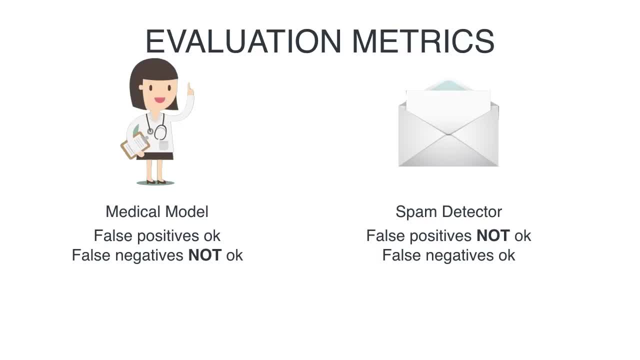 model and the spam detector model are fundamentally different. right in the, the medical model is okay with false positives, but not okay with false negatives, whereas the spam detector is not okay with false positives and it's okay with false negatives. so, in principle, the medical model is is trying. 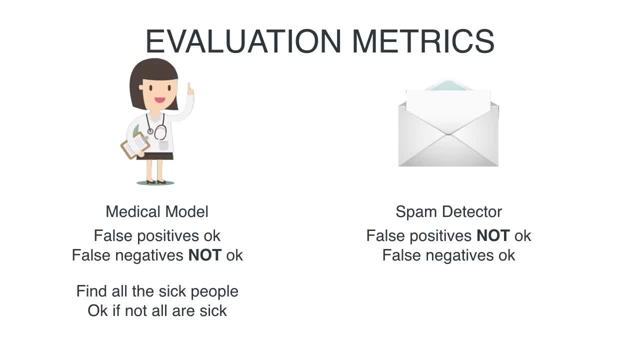 to find all the sick people and it's okay. if it finds some extra people, it's fine, whereas the spam detector says: well, I don't necessarily need to find all the spam, but whatever I find it better be spam. so we call the medical model a high recall model and the spam detector a. 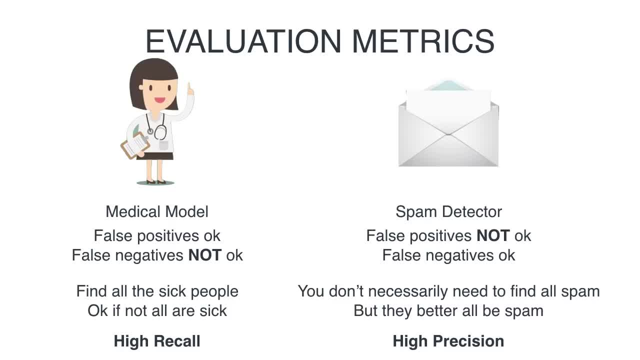 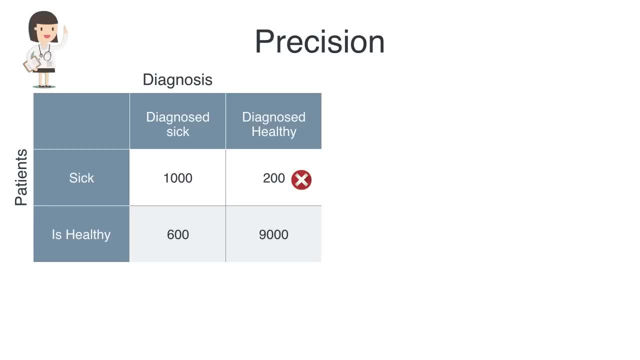 high precision one. those are the two metrics that we're going to measure: recall and precision. so let's define precision, okay, and I'm put- I have an X there, because that's what we really really care about- right, the sick people that are diagnosed healthy, that's. that's the 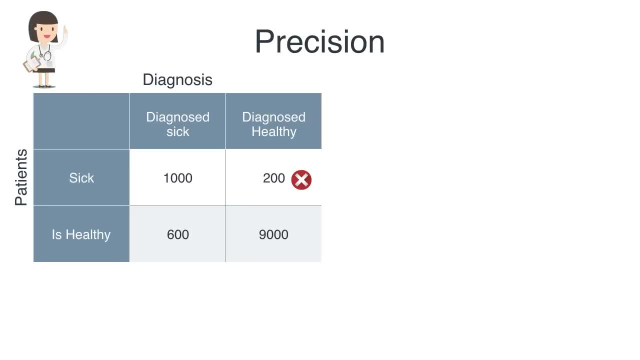 the number that we're trying to avoid. so precision answers the following question: out of all the patients that we diagnosed with an illness, how many did we classify correctly? okay, so precision is this row, because this row are the ones that we diagnose as sick, so it's a thousand that were correct, versus 1800, which is the ones we diagnose as sick, so it's 55.7. 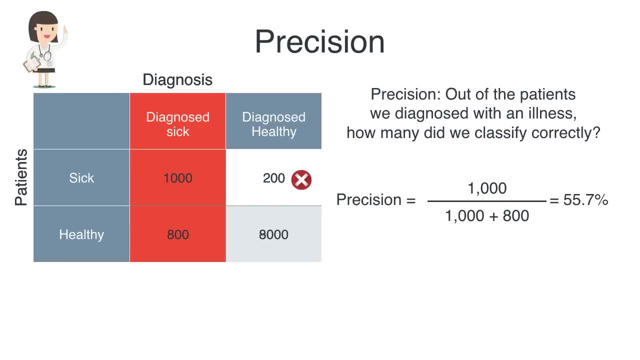 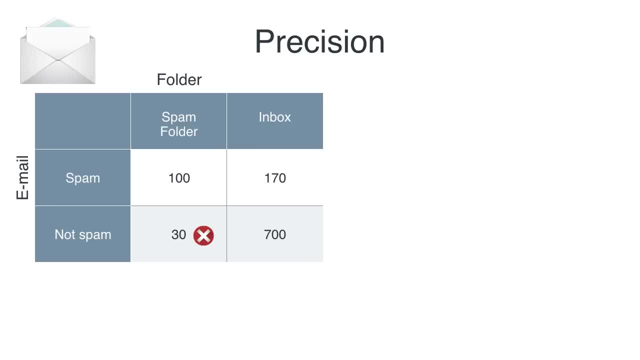 is not a very precise model, but again, we're avoiding that red x, so that's, that's okay. what is the precision of the spam detector model? so see, the red x now is on the on the on the bottom left, because that's that those 30 are really bad. that's where we want to avoid. 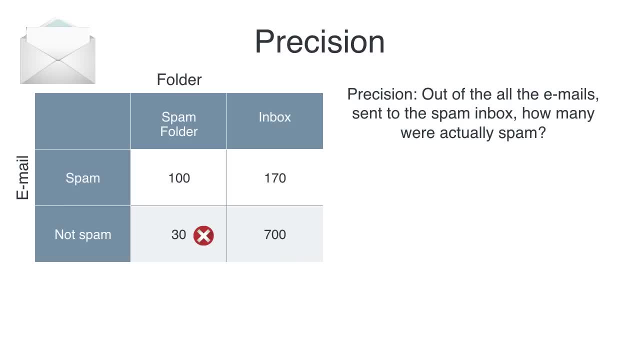 so again, precision says: out of all the emails sent to spam box, how many were actually spam? so again, this column is precision. so it says 100 that are correct you divided by 130. So this model has 76.9% of precision. and then this model needs high. 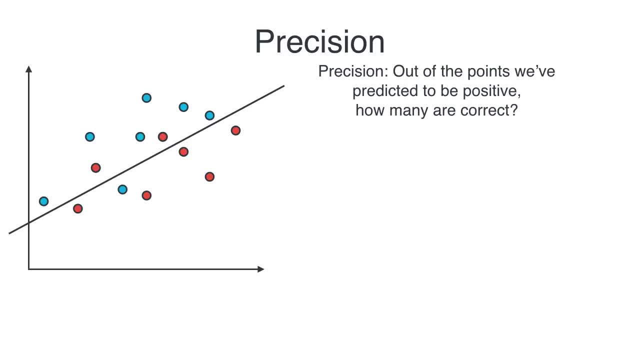 precision. So that number better be big. Let's go to our linear model. What about here? precision Of all the points we've predicted to be positive? how many are correct? So let's take a few seconds to think about it. So the points that were predicted to be positive. 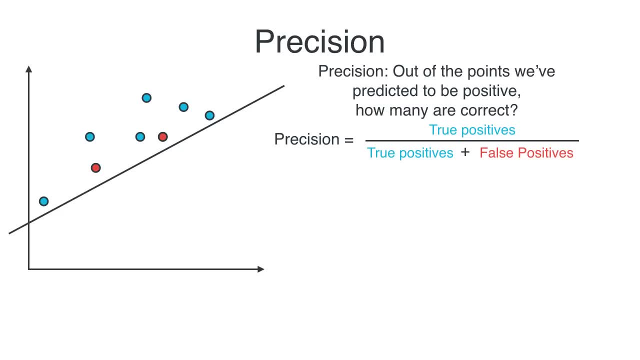 are only these ones, so we only need to focus on these. And now, precision is the number of true positives divided by the number of true positives plus false positives, So it's the ones that are correct. which are these six divided by all of them, which are six? 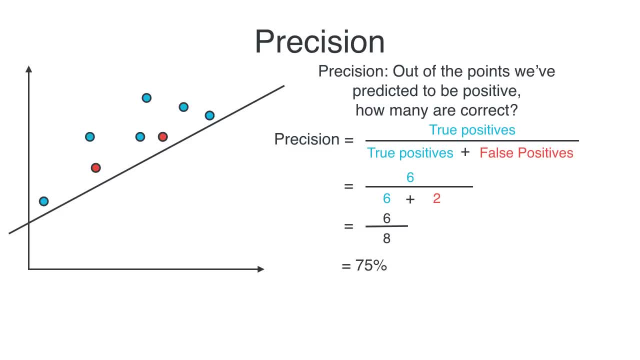 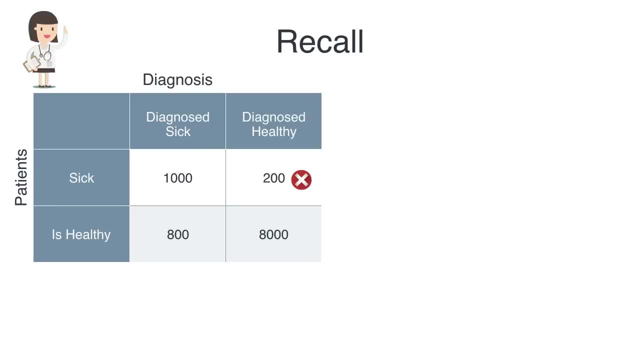 plus two, which is eight. So this precision here is 75%. Okay, Now let's look at the second metric, which is recall. So recall in the medical model, recall is answering the following question: Out of the sick patients, how many did we? 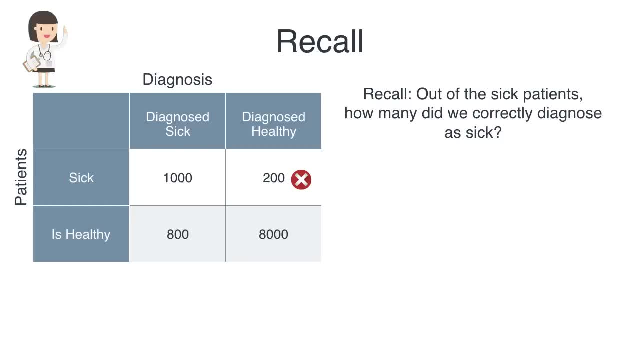 correctly diagnose as sick. So remember, precision was out. of the patients we diagnosed as sick, how many were actually sick? Now, recall is: out of the patients that are sick, how many did we correctly diagnose as sick? Now, this is this row and this row is grabbing that. 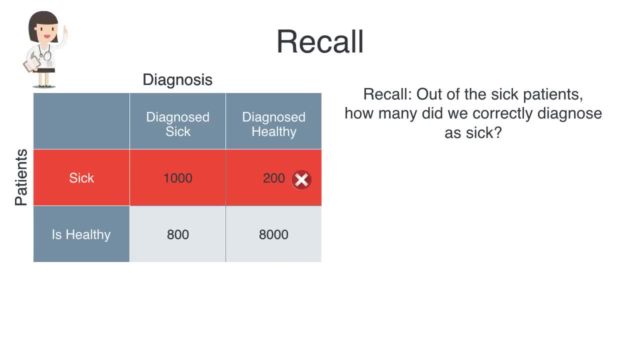 red X. So this is this. We see that this is an important metric for this model. Recall is from the 1200 sick patients. how many did we diagnose correctly? Well, a thousand of them. So a thousand divided by 1200, that's 83.3%. This model better have good recall because we want to catch. 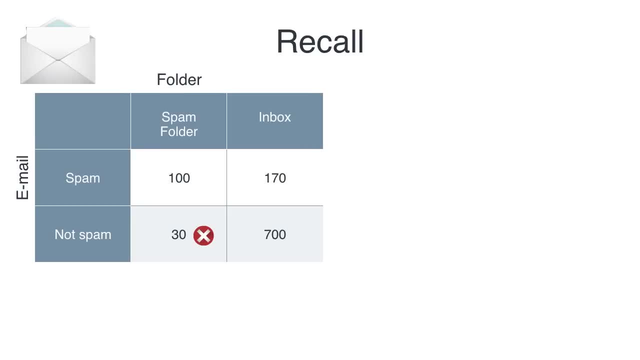 all the sick people And the recall of the email model. well, is saying how many out of all the spam emails, how many were correctly sent to the spam folder. It's this row over here. So we have a hundred correctly sent to spam folder divided by 170.. It's a very low recall. 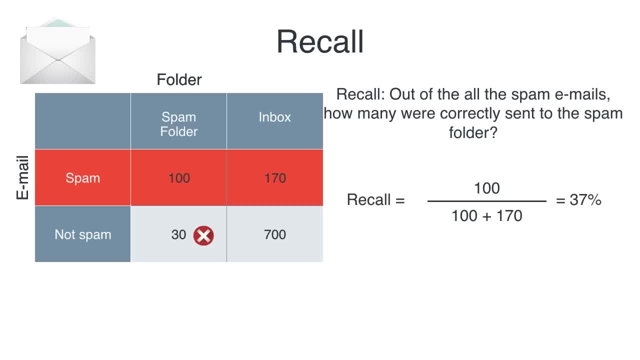 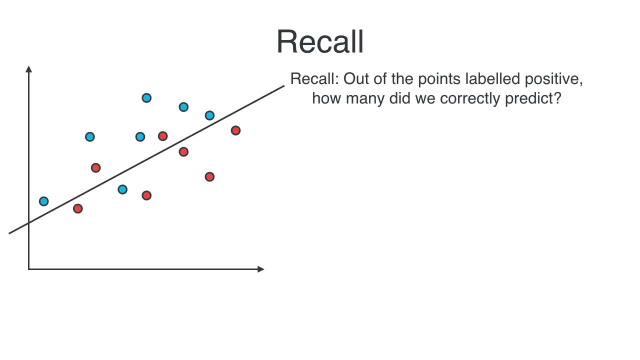 But again we're worried about avoiding that red X in the bottom. So this model doesn't need to have high recall. And again, linear model. Let's see how it's doing with the recall. So it says: out of all the points labeled positive, how many did we correctly predict? So which? 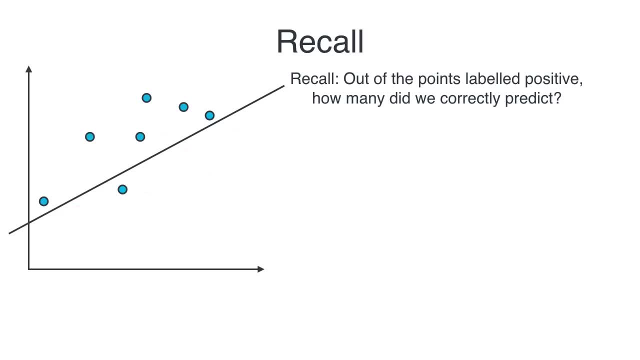 points are labeled positive, The blue points, And so recall is true positives. So how many were correct, Correct among these, divided by all of them? So it's six divided by seven. six plus one And six divided by seven is 85.7%. So that is precision and recall. So that's a summary. 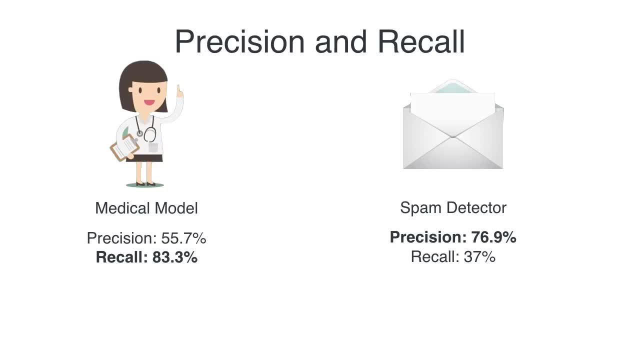 we have that for the medical model the precision is low, it's 55.7%. The recall is high at 83.3%. This is a model that's supposed to have high recall. And for the span detector model the precision is 75.3%. It's 85.78%. So that's seeing if these records are good. 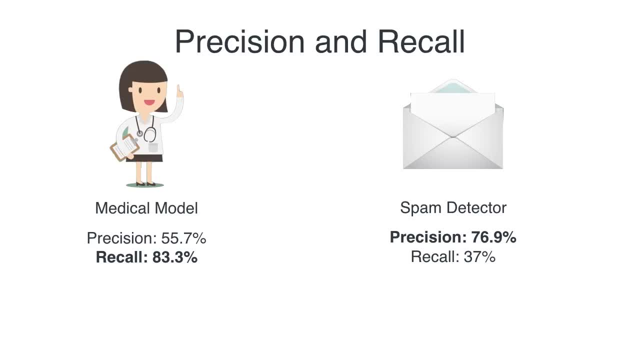 is 76.9 percent and the recall is 37 percent, but the spam detector model is supposed to have high precision. now the question is: do we want to be carrying two numbers around? do we want to be carrying precision in one pocket and recall in another pocket, and always looking at both? 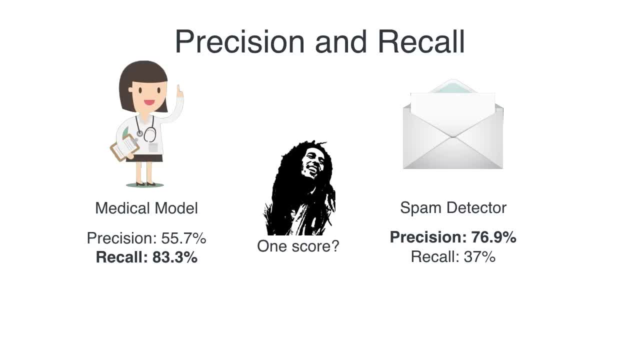 we kind of want, uh, to have just one. we have. we want only one score, right. so how do we combine these two scores into one? can you think of a way? well, a pretty simple way is is taking the average right. so let's take the average of precision and recall. so on the left we get 69.5 and on the right 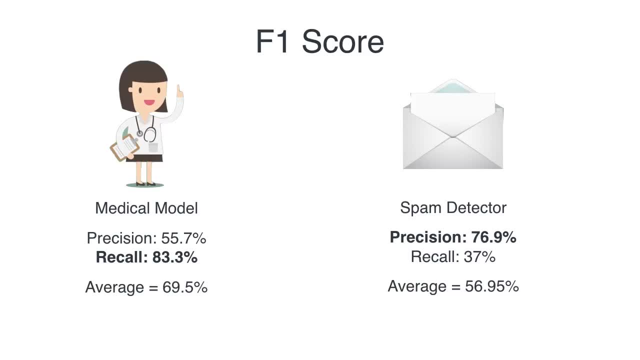 we get 56.95 and that's, that's an okay metric, but i'm sure you're probably thinking in your head it's like that's not much different than than accuracy. right, that's, it's not telling too much. okay, and the way to see what what this average means and how it's doing is to try it in the extreme. 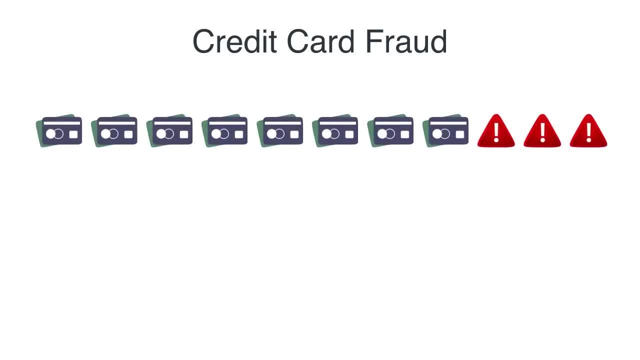 example. so the credit card fraud example. so again, we have some good for credit card transactions and some fraudulent ones. these are how many we have, and let's pick our terrible model, number one, which says all transactions are good. so what's the precision? well, the precision is out of the 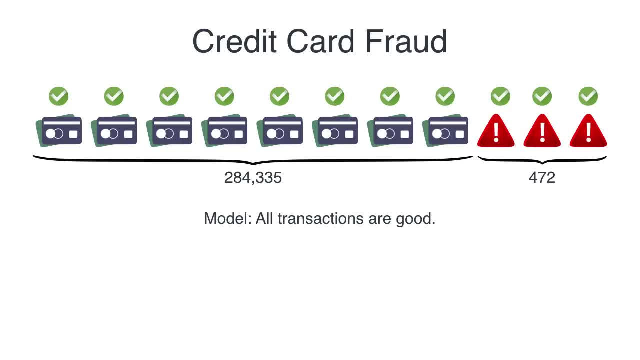 ones we classified as bad. how many are bad? that's a hundred percent, because technically we never didn't classify them as bad. so we're going to classify them as bad and we're going to classify anything as bad. uh, now, what about the recall? well, the recall is: how many of the bad ones did we catch? 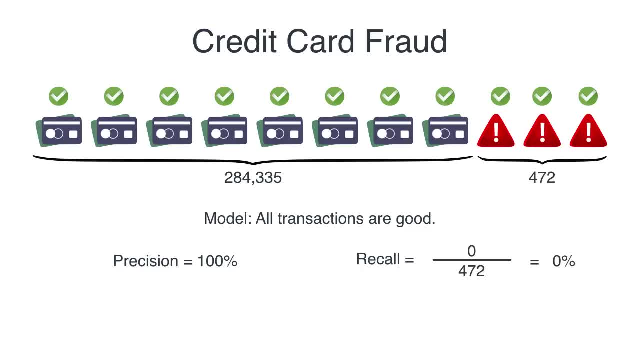 and that's zero because we didn't catch anybody. so zero percent. so the average between precision and recall is 50, so the average between 100 and zero. now the question is, do i want to give that horrendous model a score of 50? it seems like a very high score for such a bad model. 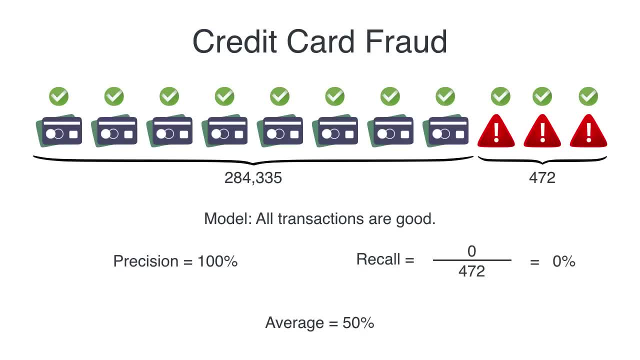 so i kind of want to give it a zero. so average is not that good. let's try the opposite. let's try the model that says that all transactions are fraudulent. what's the precision of this model? well, i correctly diagnosed 472 out of all of them, so it's 0.16 percent, and the recall is i caught? 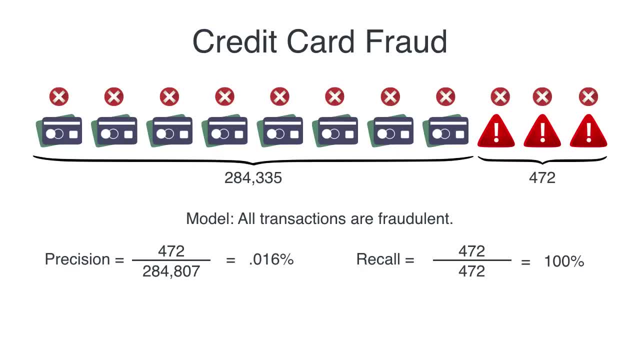 all of them. so actually pretty good recall: it's 100 percent. what's the average within between precision and recall? well, it's slightly over 50 percent. uh, again a terrible model with a 50 score. that's not good. i kind of want to give it a zero too. so average seems like it's not the 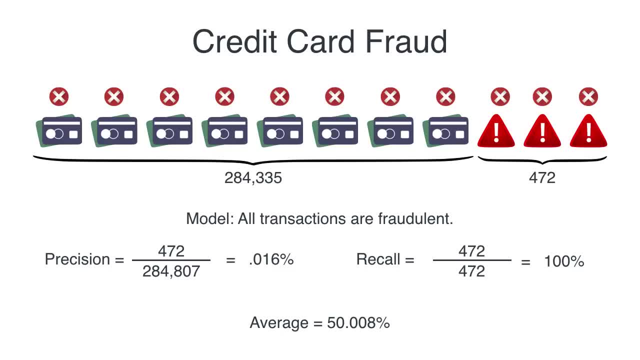 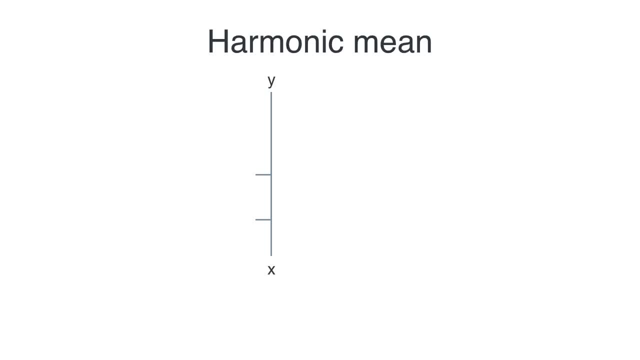 greatest thing. but there's another kind of type of average that we can learn, and this is called a harmonic mean. so let's say we have two numbers, x and y. x is on the bottom, y is on top, and we have the arithmetic mean. here it's x plus y divided by 2, and there's something called the harmonic mean. 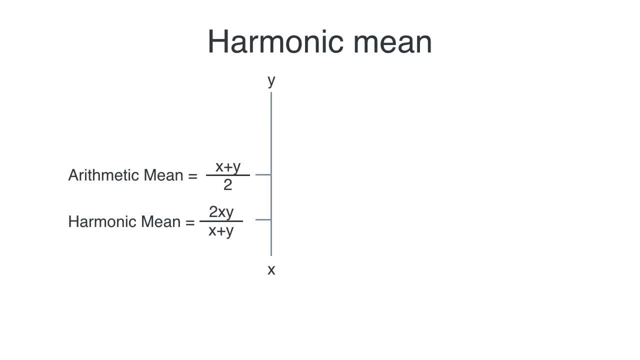 which is defined as 2xy divided by x plus y, and it's kind of an average too, uh, in the sense that if, if the numbers are equal, if x and y are equal, we get. we get x or y, but it actually it's a mathematical fact that 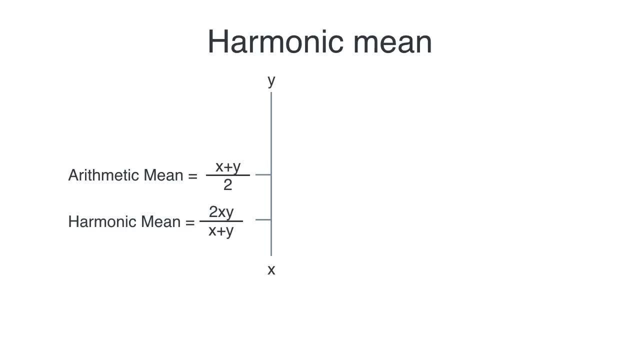 it's always less than the arithmetic mean, so it's kind of closer to the smaller number than to the higher number. let's look at an example: if my precision is 1 and my recall is 0, my average is 0.5, the harmonic mean. if you plug it in the 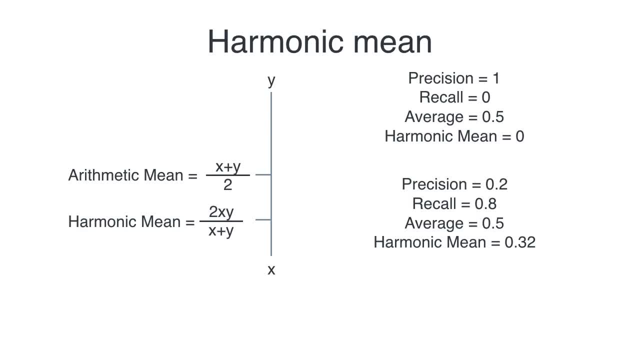 formula, you actually get zero, uh, if my precision is 0.2 and my recall, 0.8. again, the average is 0.5, but the harmonic mean is uh 0.32. okay, so we're not going to use the arithmetic mean, we're going. 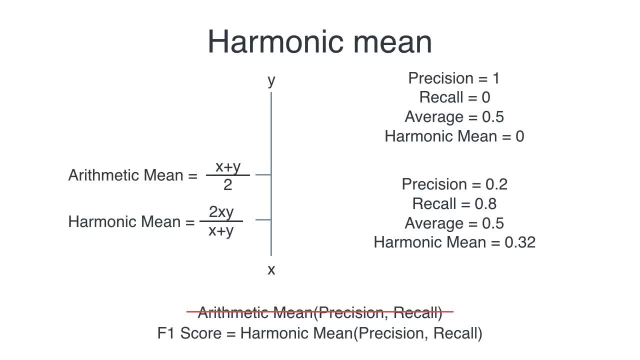 to use the harmonic mean and that's going to call the f1 score. uh and uh, as, as we said, the f1 score is closer to the smaller one. so if, if one is small, between the heart, that between the precision and recall, the f1 score kind of raises a flag, whereas the the average kind of like says if one is bad. but 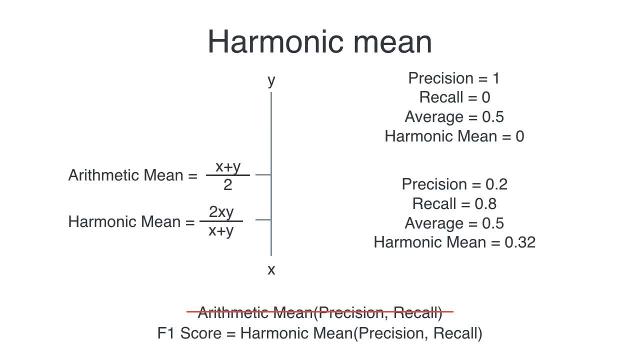 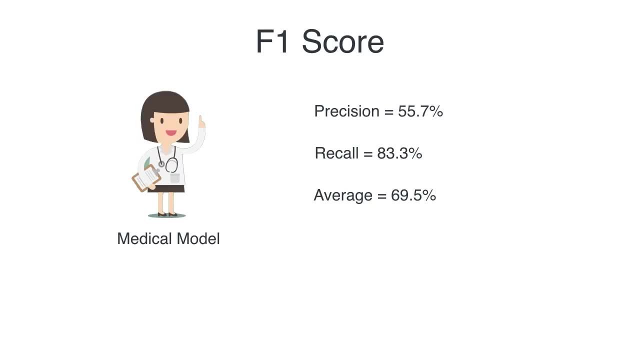 the other one is good then i'm so. so, and that's why we're going to use the f1 score more. so let's see what the f1 score is for our medical model. so our precision is 55.7. our recall is 83.3. 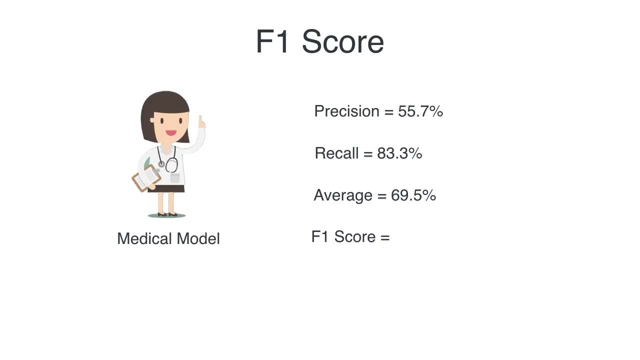 our average is 69.5, and then the f1 score is just this formula over here, which ends up being 66.76, and for our span detector model precision 76.9 recalls 37 average 66.95 and the f1 score. 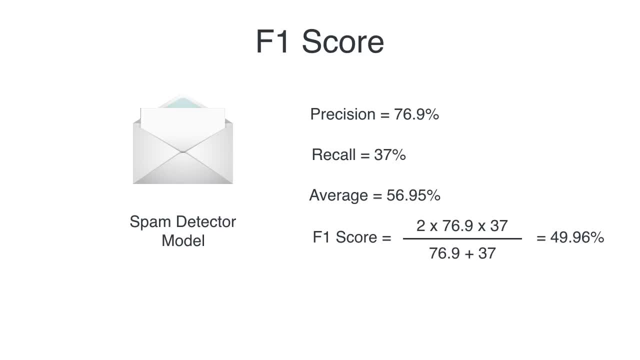 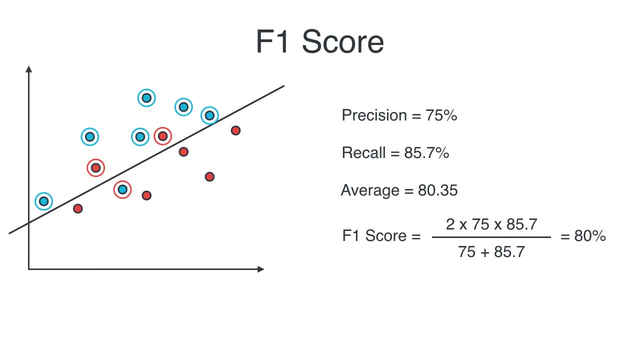 is this formula which gives us 49.96. and finally, for a linear model: precision 75, recalls 85.7, average is 80 and the f1 score is this formula, which is 80 percent. that one looks like a little lame because the precision or recall are very close, so the average and the f1 score are very close too. 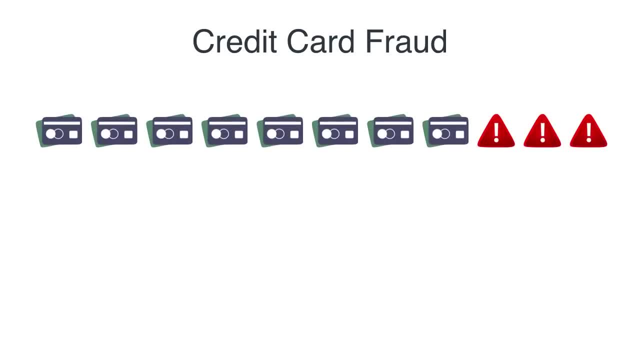 now let's look at precision recall for our credit card fraud example. so the bad model that says all transactions are good gets 100 precision, zero percent recall. f1 score is actually going to be zero if you plug in the formula and there's actually something more general than f1 score. it's called the f beta score. 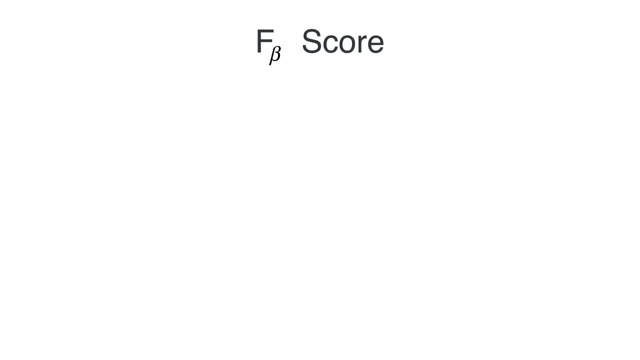 and it's kind of like a. the beta is any number that is higher than zero and if the beta is one means you're you're taking the, the harmonic mean between precision and recall. but if you're taking, if your beta is small, then you wait more on precision, and if your beta is large you wait more on recall. 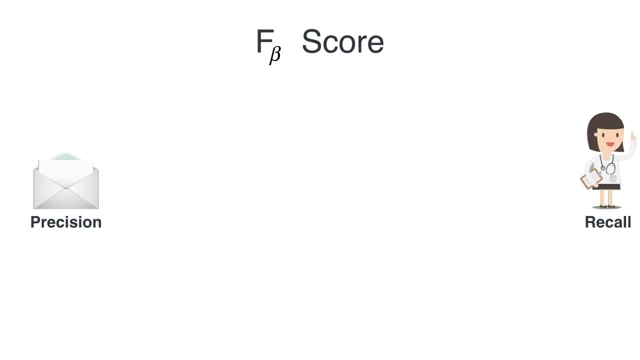 so if precision is over here for a spam model and recalls over here for a medical model, f1 score is kind of in between. f0.5 score is closer to precision and f2 score is closer to recall. uh, question: where would the credit card fraud model be? uh, where? 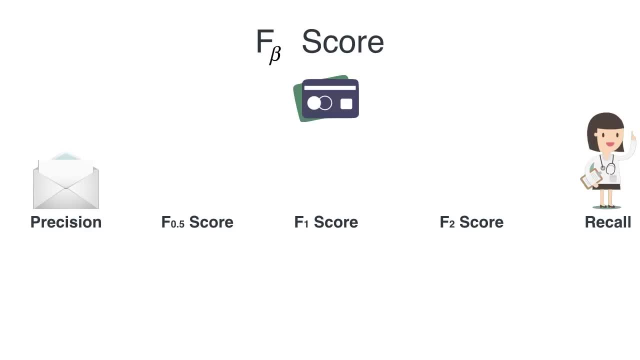 where would the credit card fraud model be where? what would be a good metric for it? closer to precision or closer to recall? so i'll let you think about it for a moment. well, the question is: what do we prefer? do we prefer to catch all the fraudulent transactions, or do we prefer that everything? 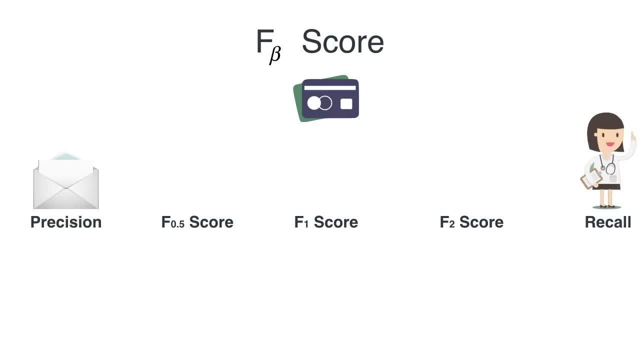 we catch is a fraudulent transaction. so what's worse? if you accidentally get a text saying your transaction may have may have been fraudulent, check this out. or if a fraudulent transaction happens and the model that you're using is fraudulent, check this out. or if a fraudulent transaction is a fraudulent transaction, it still doesn't catch it. so, in my opinion, the the second. 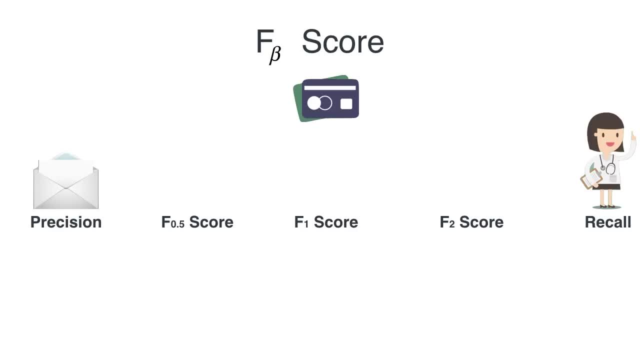 one is worse. i don't mind getting the occasional text about a fraudulent transaction that i have to make a call and approve, but i really do mind if there's a fraudulent transaction done on my credit card and it's never caught. so this, the good score for this one, is going to be over here pretty close. 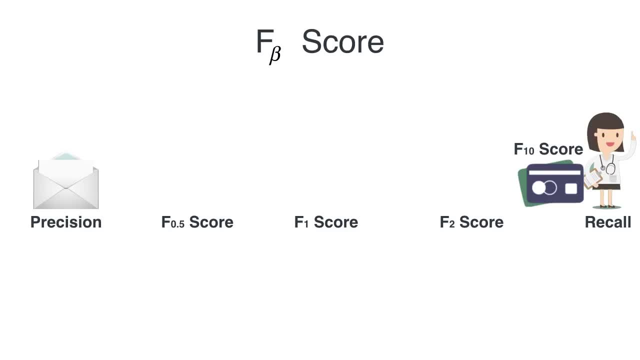 to the recall. let's say maybe f10 score, uh, and in general that's a good way to to analyze our models, to say what do i want more precision or recall, and then, with that score i'm going to be in mind, we pick a number for the F, for the F beta score that that resembles. 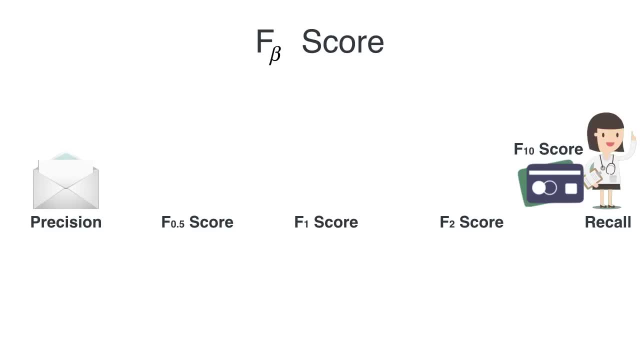 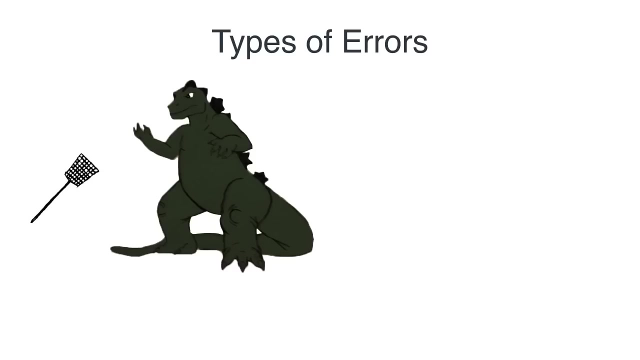 that okay. so now that we've seen some metrics, let's go to a different topic. the different topic is the types of errors that we can make when we train a model, so, like in life, there are two types of errors we can make right. one is if we try to kill Godzilla with a fly sweater. the other one is if we try to 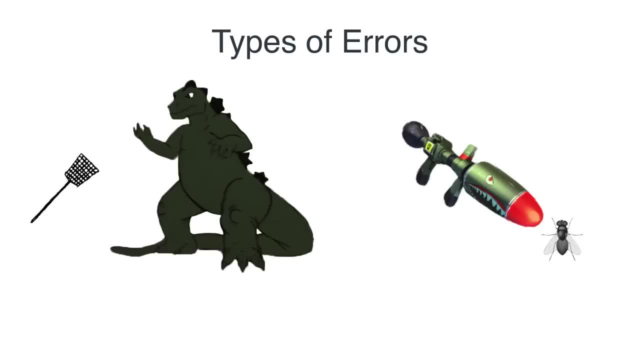 kill a a fly with a bazooka. so there are two different types of errors. right, that the left one try to kill Godzilla with a fly sweater. it's kind of over simplifying the problem. right, it's underestimating the the size of our problem that's called under fitting, and the one on the right which is trying to. 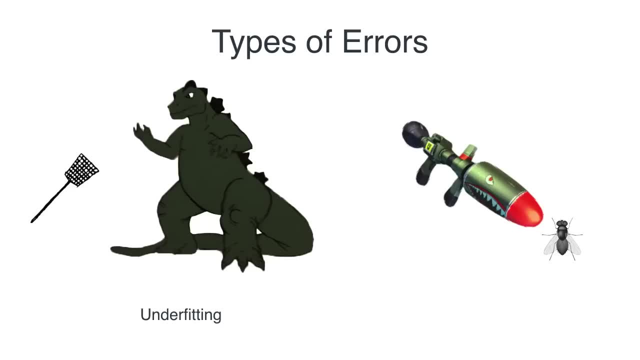 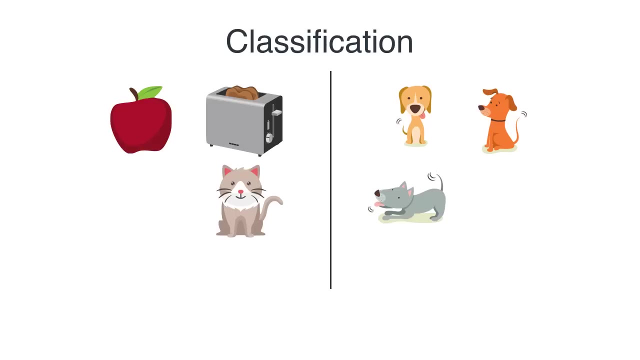 kill a fly with a bazooka is the opposite. is is completely over estimating our problem, and so that's called over fitting you. so let's look at a classification problem, and the classification problem is this one. so what does it seem like that the rule here is for, for, for. 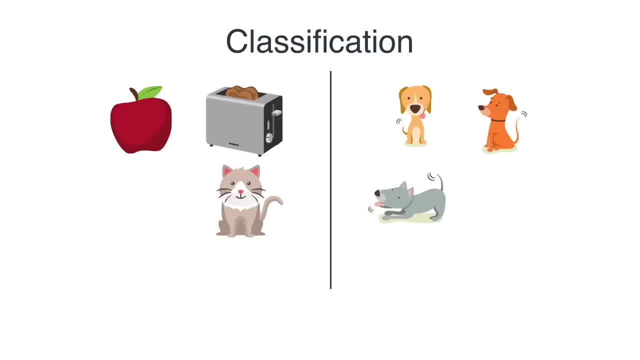 classifying the data on the right and on the left, like you think about it. well, it seems like a good rule is: on the right we got dogs and on the left we got not dogs. so that's. that's a pretty good model, right? what if we said the following: on the right, we have animals and on the left we 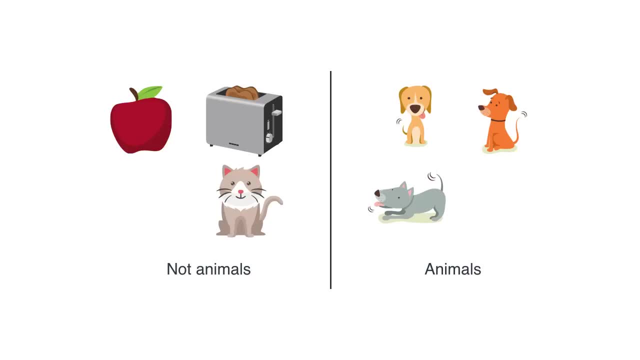 got things that are not animals. what's wrong with that model? what's wrong that model is that the model is too simple, right, where we're underestimating the problem. we're not even correctly classifying the training set, because here's an error. right, we got a cat and we classified us, not an animal. but 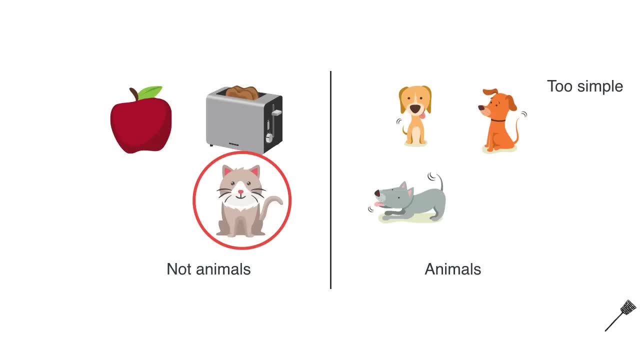 that's an actual animal. so so this is- we're kind of like simplifying the problem too much, where we're underestimating our data, and that's like killing a trying to kill Godzilla with a fly swatter- right, that's, that's underfitting. we're also gonna call it error due to bias. now, what about the? 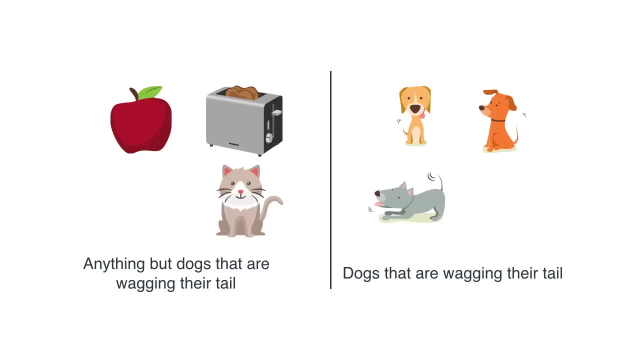 following for the following model now, on the right, we have dogs that are wagging their tail and on the left, we have anything but dogs that are wagging their tail. what happens with this, with this model? well, the model does pretty well in the training set because- check it out- everything in the right is correctly. 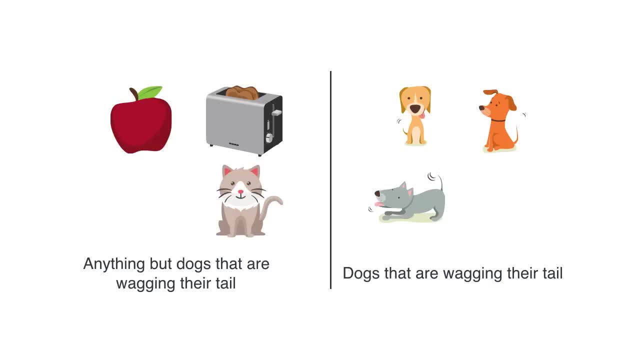 classified and everything left is correctly classified. but what's the problem if we get a testing point, it's this dog. where does this? where does this point fit? it kind of fits in the right with the other dogs, but the model says it's gonna be on the left because it's actually not wagging its tail, so it's. 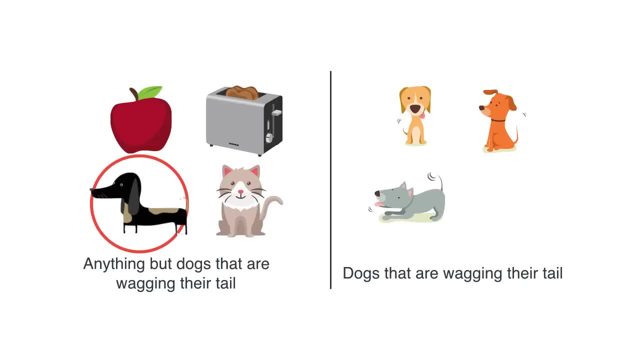 models making a mistake. so what is wrong with this model? well, it's way too specific, so it kind of memorizes the data instead of really catching a good rule, and that's, that's um over complicating our problem, which is like killing a fly with a bazooka, so that's. 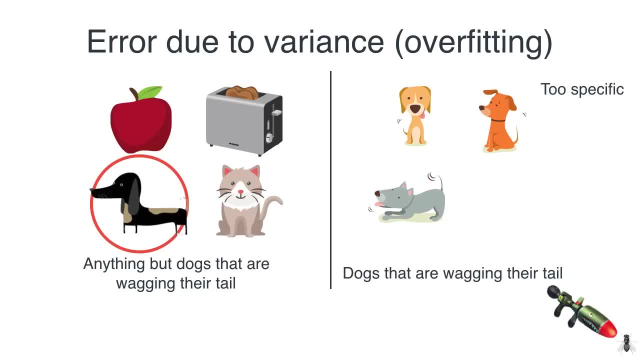 gonna be called overfitting or error due to variance. okay, so those are the two types of mistakes we can make: error due to bias or underfitting, or error due to variance or overfitting. let's look at how they work with some data. so let's. 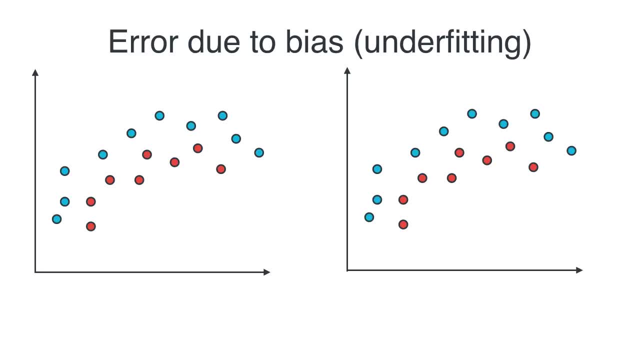 look at this data that's here twice. it looks like the answer is kind of this: right, it's a quadratic equation that separates the red points and the blue points. what if I were to think that a line can do it? so a line is a much simpler solution. that doesn't seem like. 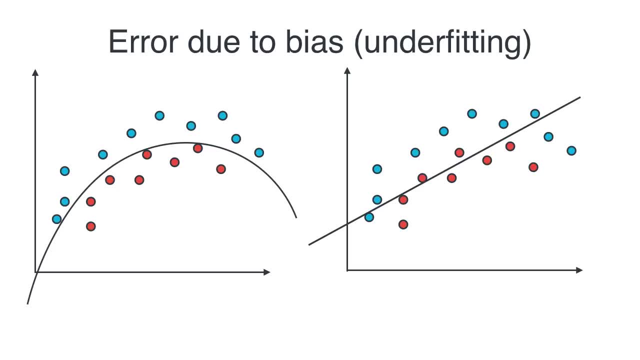 the right answer and it makes a bunch of mistakes. and the mistake we make here is that we kind of oversimplified it. we try to solve a problem that is inherent, inherently quadratic, with a linear equation, so we underestimated the data we did, underfitting 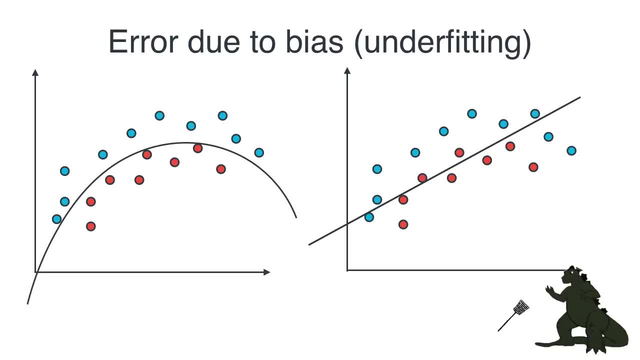 which is like trying to kill Godzilla with a flyswatter. What about this? We have the data like this and again, the right model seems to be a quadratic equation that separates the red points from the blue points, but instead we're going to look at: 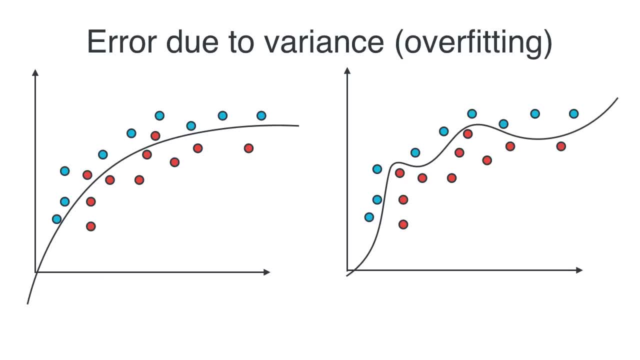 a super complicated high degree polynomial that fits our data pretty well, but, as we saw in the beginning of this video, that's not a good solution because, even though it does fit the training set well, it will not generalize well, so it doesn't really learn. 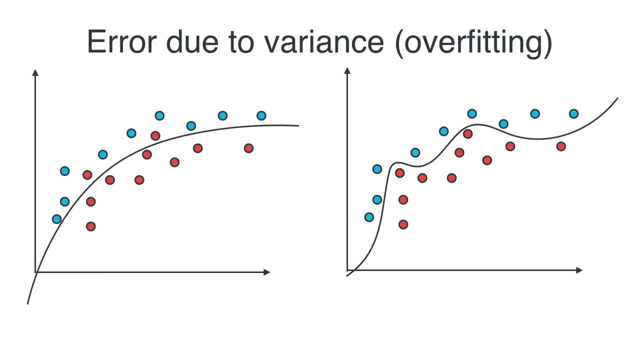 a good model. it just memorizes the data, so it's overcomplicating the solution and that's overfitting, so it's like trying to kill a fly with a bazooka. So let's look at the three little bears. 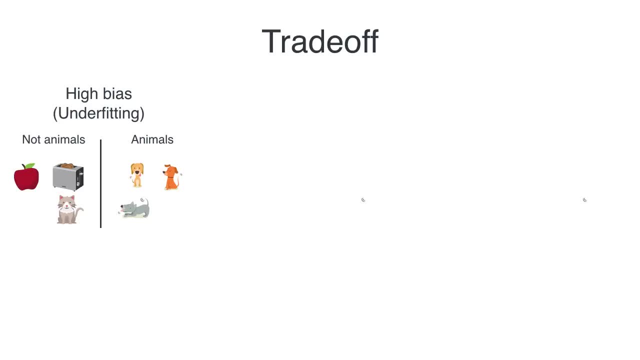 On the left, we have a v, Very, very simplified solution that underfits. On the right, we have a very, very complicated solution that overfits, and in the middle we have just right. Just right. it says dogs and not dogs seems to be the right way to classify this data. 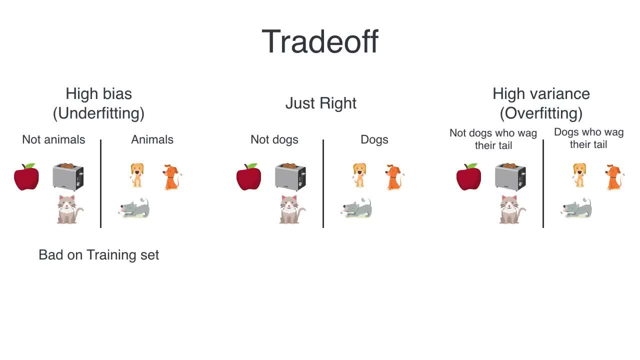 So what happens with the one on the left? Well, it's bad on the training set because it makes a mistake on the training set. that cat gets it wrong. On the other hand, the complicated one is great. It's good on the training set. it fits it really well. 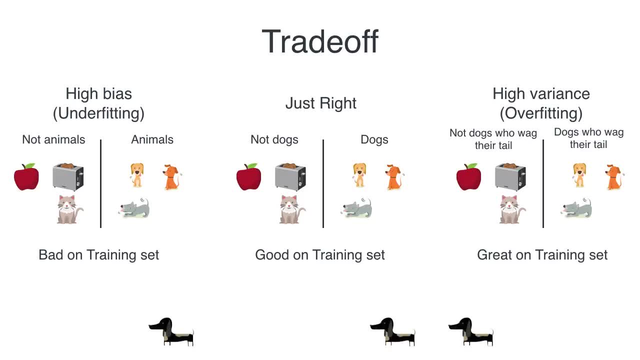 And the one in the middle is good on the training set. What happens if we bring a testing set? Well, the left one is bad on the testing set as well, because if it's not good with the training set, even the testing set is worse. 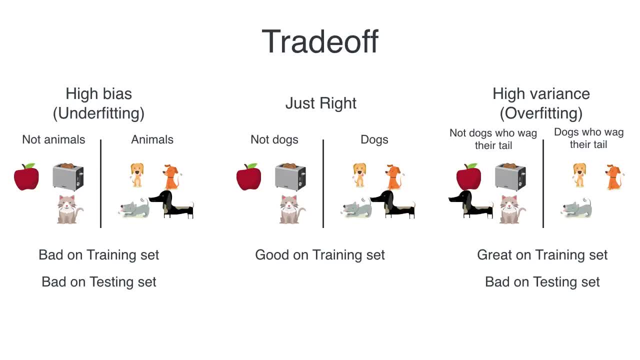 So here it correctly classifies the dog, but that doesn't mean anything. The one on the right is bad on the testing set because it incorrectly classifies a dog, whereas the good model is good on the testing set. So that's how we tell them apart. 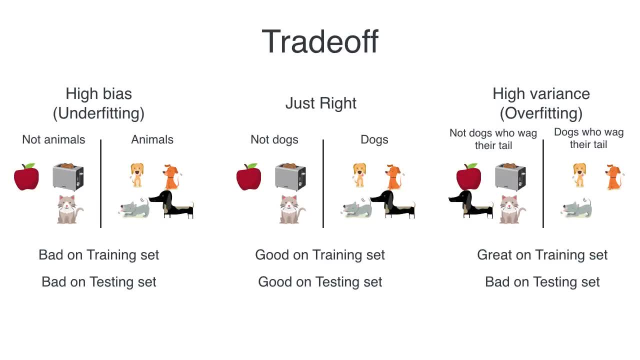 If you have a model that is bad on the training set and bad on the testing set, you have underfitting. If you have a model that is great on the training set but terrible on the testing set, you have overfitting. 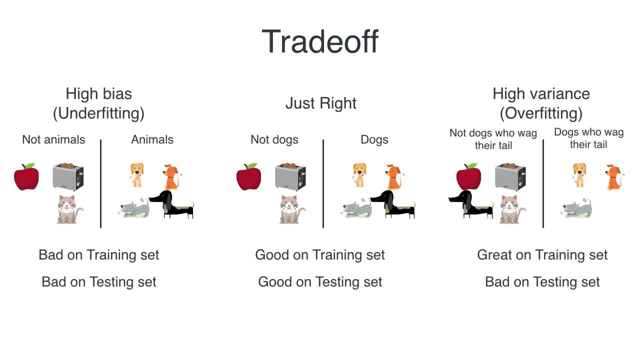 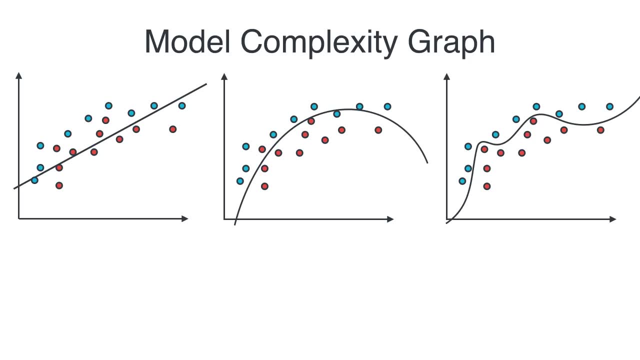 And you want something that's good on both the training and the testing set. So let's take that last observation and make a graph out of it. It's called the model complexity graph. So again we have the three little bears. On the left, we have a high bias solution. 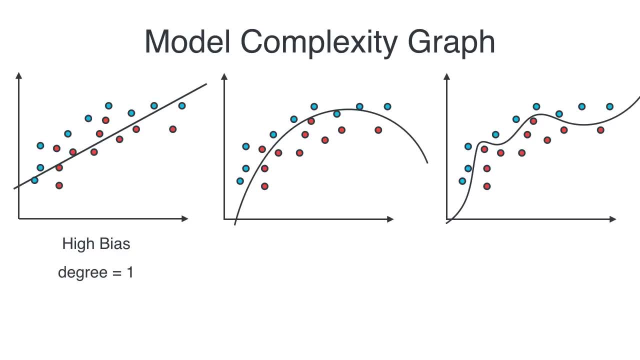 This is underfitting, which is trying to fit a degree WAM polynomial on data that is clearly quadratic. On the right, we have the overfitting or high virus, which is thinking that the solution is degree six when it's really degree two. 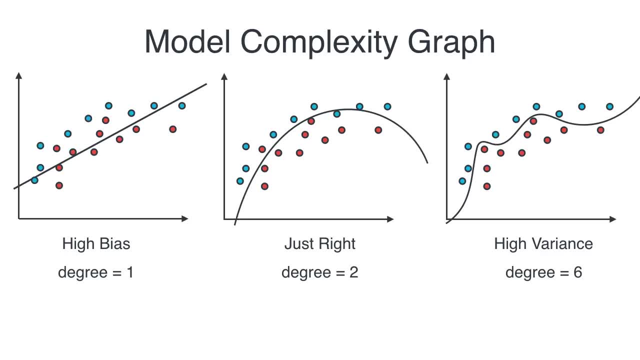 And on the middle we have just right, which is the degree two solution to a problem that is inherently a degree two problem. On the left, we have underfitting, killing Godzilla with a fly swatter. On the right, we have overfitting, which is killing a fly with a hijack. 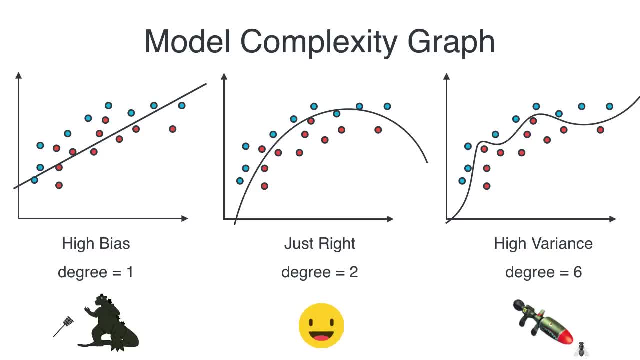 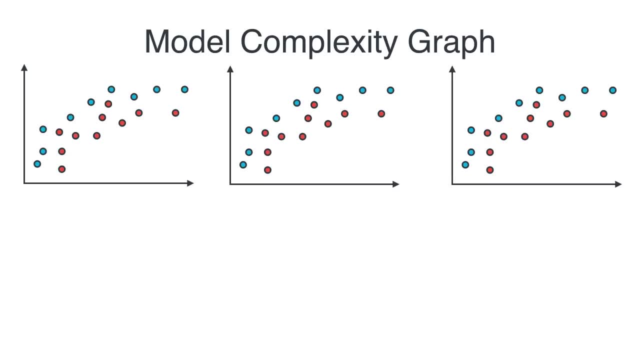 Some thought the problem was based on the scientific results, which we will cover in a video in a moment, with a bazooka and on the middle we have just right, so we're happy. so, as promised, we're going to turn this into a graph. so again we have our three little bears: the degree one, degree two. 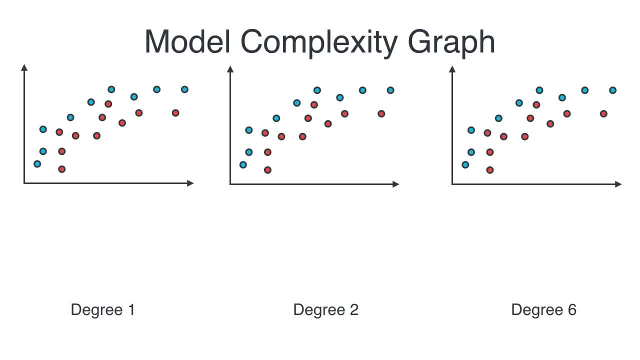 and degree six, and let's recall that from the beginning that we uh, we had the training set and the testing set- separation on the data. so here we're going to take the colored points as the training set and the points that are empty in the middle as the testing set, and we're going 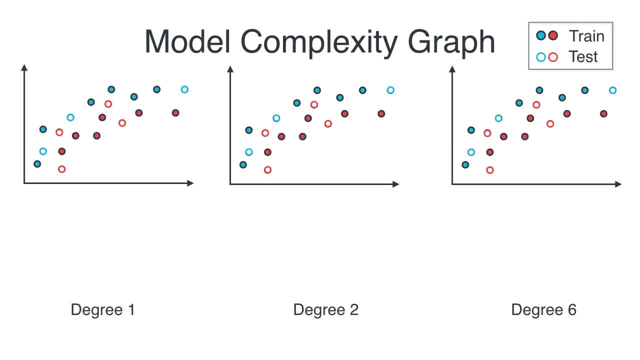 to build the three models and look at their training and their testing errors. so let's build the first model. that's a line, and the question is: how is it doing on the training set? well, it's making three mistakes. they're highlighted in green, so the training error is three. and now let's see. 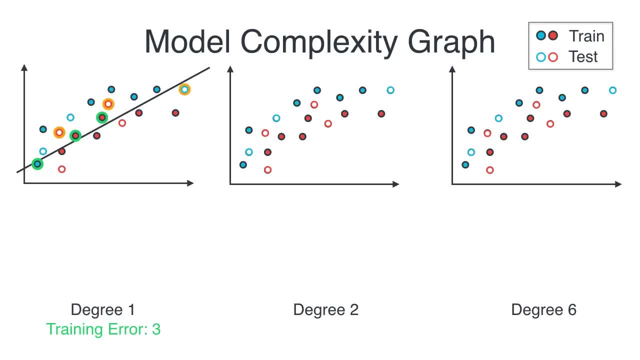 how it's doing on the testing set. so it's making three mistakes on the testing set. these are the yellow highlighted points. so the testing error is 3, so let's put it on this grid: training error is 3, testing error is 3, training is green, testing is yellow and. 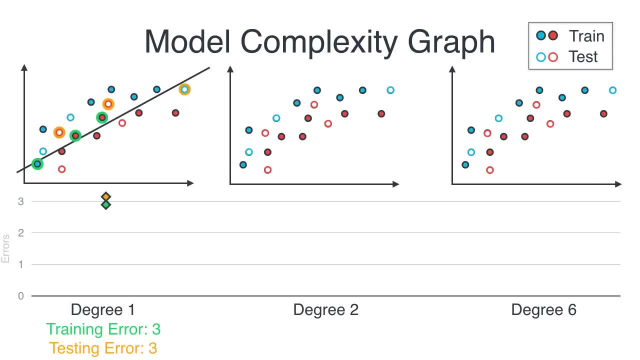 now let's do the same on the other two models. so on the on the second model, the degree 2, we fit our polynomial. how did it do? well, it made one training mistake. this point over here. and it made one testing mistake. so this point over here. 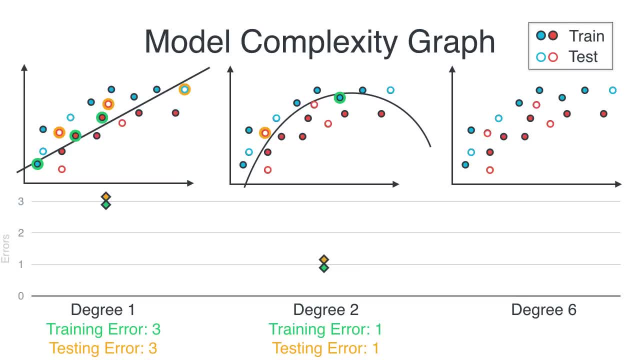 so the training error is 1 and the testing error is 1. now let's look at the complicated degree 6 model. how did it do in the training error? well, by nature, overfitting models do very well in the training error, so it did very well it. 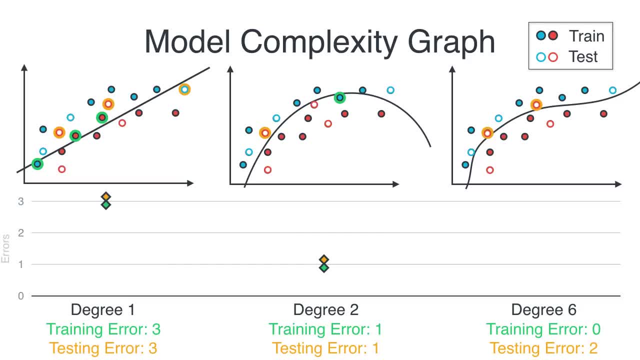 made no mistakes. how did it do on the testing set? well, it made two mistakes. so our training error is 0, our testing error is 2. so we can see that the it's the rule that we said at the beginning, right under fitting problems are bad on training set, bad on testing set. overfitting problems are great on the. 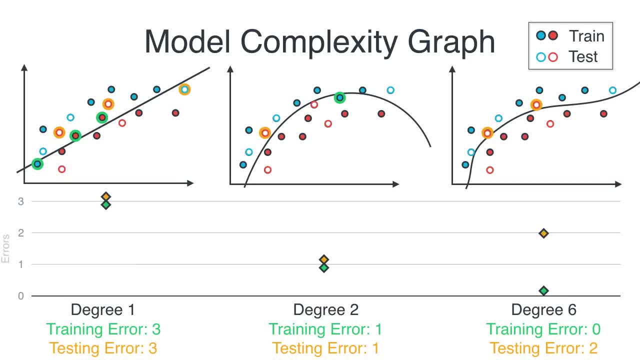 training set, but bad on the testing set and they're just right. ones are the one in the middle, which is good on the testing set and on the training set. so let's actually graph the, the curves that join the, the green points and the yellow points, and there you go. we have what's called a model complexity graph and 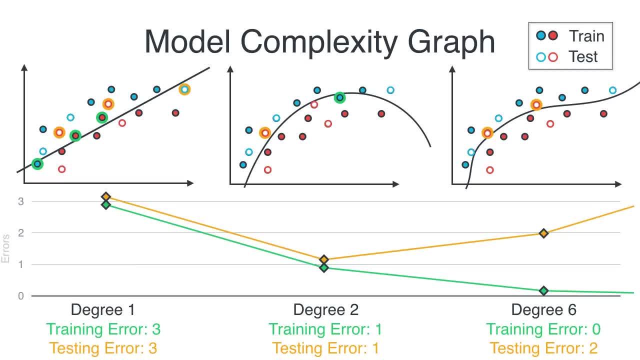 that's what we're going to call a model complexity graph, and the model complexity graph is the, the curve with the training error, which is green, and it decreases the, the curve with the with the testing error. that goes down and then up, and the way to tell where our just right model is is this: 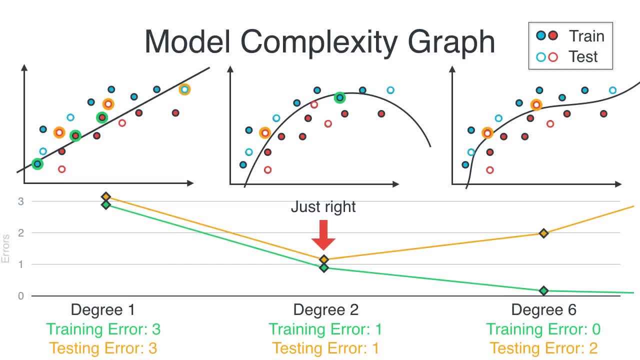 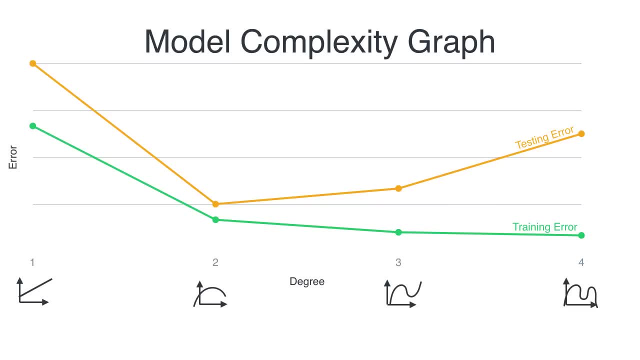 point, this point where they're the closest before starting to divert. so it looks more like this. so here we have. here we have it in a nutshell: right on the left, we have our linear model that under fits on the right, we have our high degree polynomial that under fits on the left, we have our linear model that 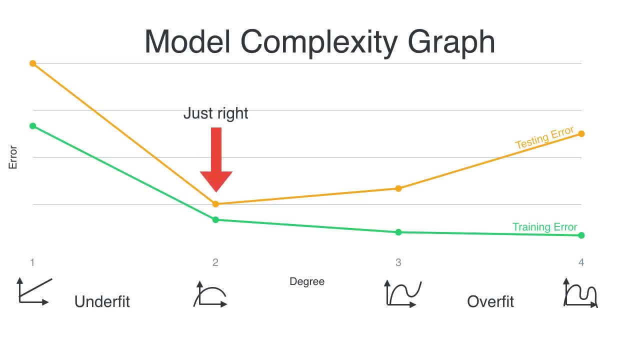 over fits, and the just right is the point here where they sort of start diverting. so very, very, very simple: what we have to do right is we have to try a bunch of models, we have to train them on the training set and then we test them. 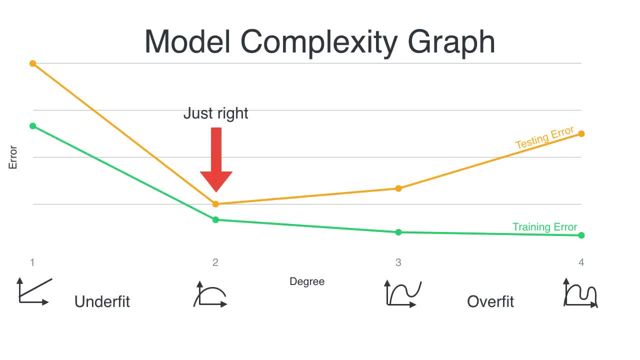 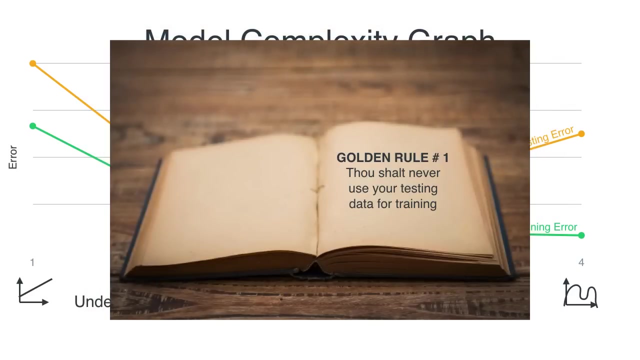 on the testing set. and how do we decide which model is better between the linear, quadratic, cubic quartic? well, we decide what model is better based on the testing error. how does that sound? it's pretty good, right? oh wait, oh no. Oh, what's happening? what is this? oh no, we did it. we broke the golden rule. this is: 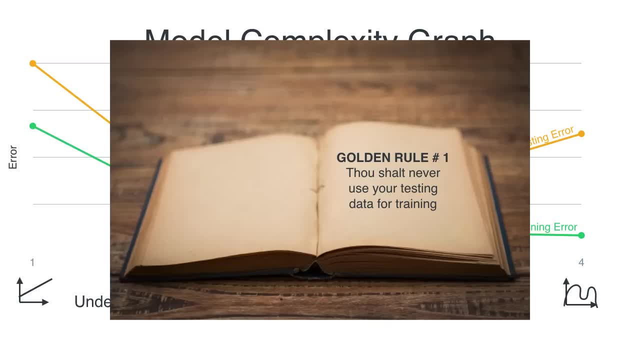 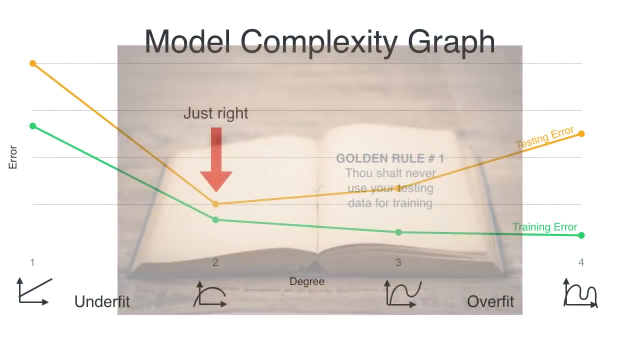 terrible though, shall never use your testing data for training. we've made a huge, huge mistake. we can't. we can't do it right. we can't make decisions based on the testing set that we have to do so free must be all right. we need to step down. 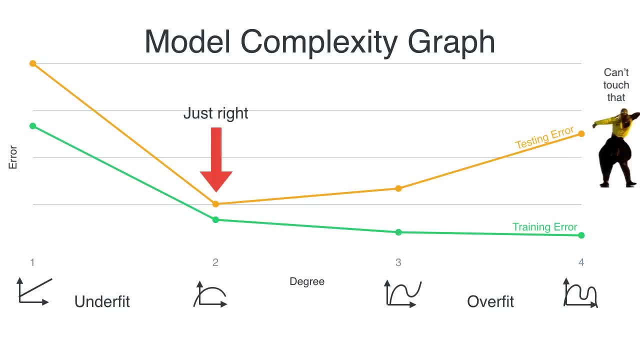 is that that? and we run. and then if we respond to test type text that says too, we, we can't, we can'tfit take seriously the testing set, we leave it at the very end: right, you can't touch that, you can't touch the testing set. so what do we do? what do we do if we can't make decisions best based on the testing set? 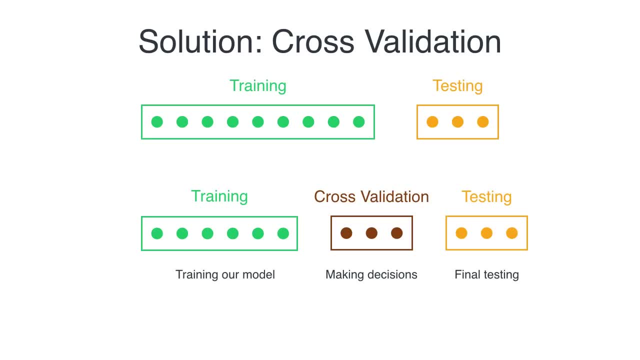 well, the solution is cross validation. so before we have training set on green, testing set on yellow. now, what we're going to do is we're going to cut a little more of our set, so we're going to take this brown set in between, so we're going to use the training set for training our models. 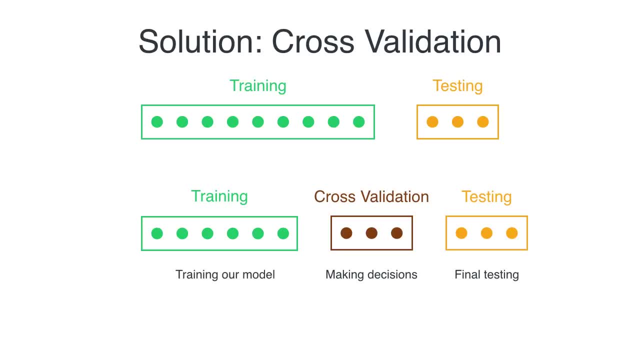 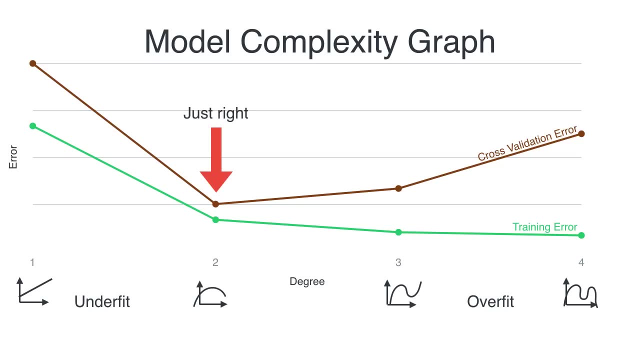 the cross validation set for making decisions such as degree etc. and the testing set at the very very end for testing. and so now this looks a lot better. we use the cross validation curve to error curve to to to decide what, uh, what, our perfect model is, and this is how it looks on the 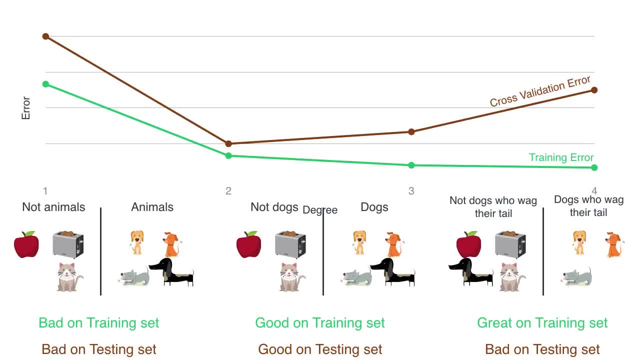 on the dog example. right on the left we have uh underfitting, so very high temperature, and we're going to use the cross validation set for making decisions such as degree testing and training errors. on the right: we have overfitting, so low training error, high testing. 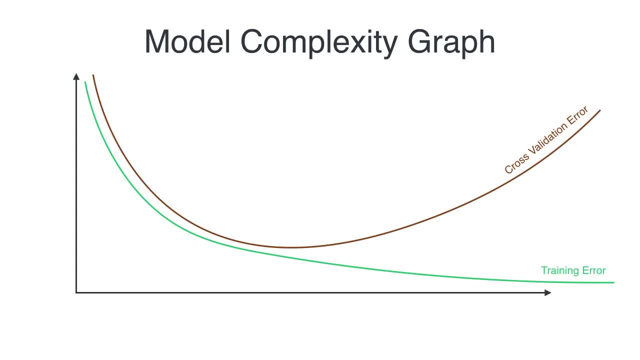 error and the just right point is here. so this is, this is kind of how it looks in in general. well, in general you may have like very complicated, weird curves, but it's kind of like this and this is, this is the just right, underfit on the left and overfit on the right. so a small summary of 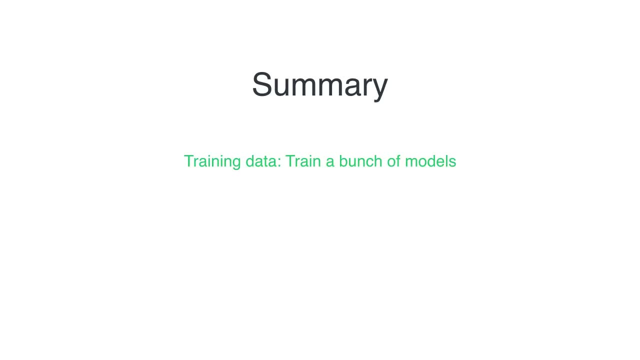 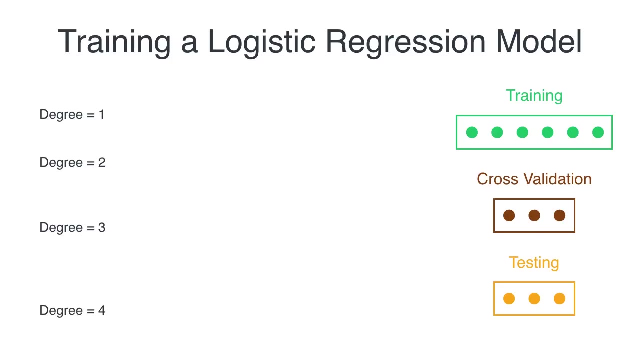 what you just did is we take our training data, we train a bunch of models and we use the cross validation data to pick the best one of our models. so, for example, for training a logistic regression model, we try a model of degree one, degree two, degree three, degree four and with the training data, we train them all. so we find the things. 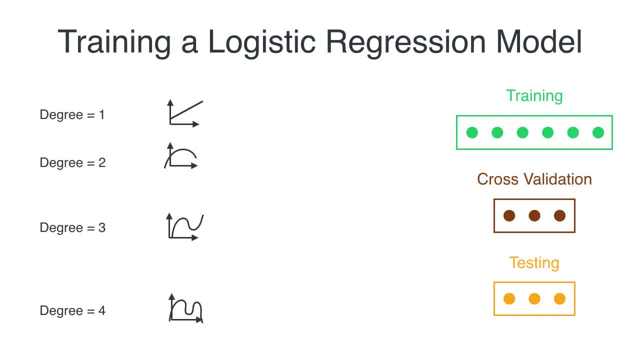 like the slope of the line, the coefficients of the polynomials, etc. then with the cross validation data, we say: pick, say the f1 score, and calculate the f1 score of all these models, and then we pick the highest one with respect to the f1 score and then, as a final step, we use: 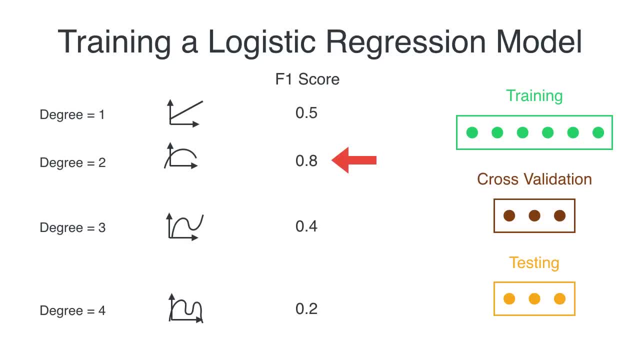 the testing data to test and make sure that our model is good. so the, the parameters of the algorithm are, are in this case the, the coefficients of the polynomial, but the degree is kind of like a higher parameter, right? so we call those hyper parameters. let's see another example. let's say 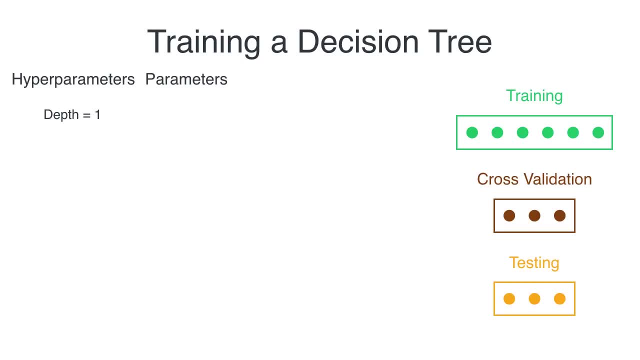 we're training a decision tree. so what are the hyper parameters? things like depth. we have: depth equals one, depth equals two, three and four. then we use the training data to take it to train a bunch of trees of depth one, depth two, depth three and depth four. so the parameters: 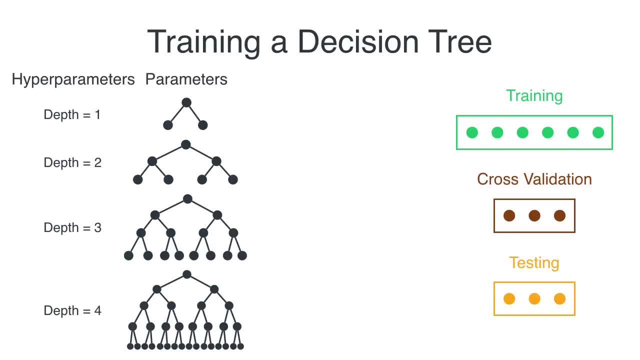 are the, the numbers in the, in the leaves and the threshold, etc. then we take f1 score and with the cross validation set, we we find the f1 score on each one of these models and then we pick the one that did better and then, finally, with the testing set, we make sure. 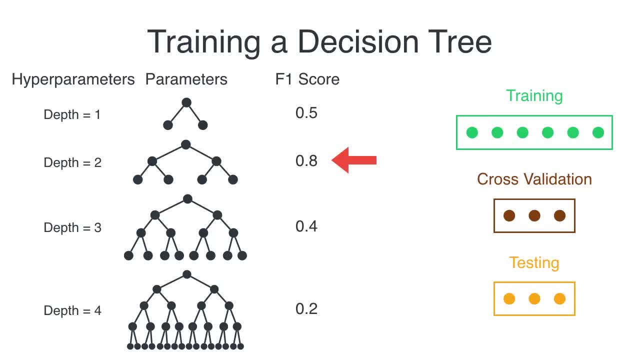 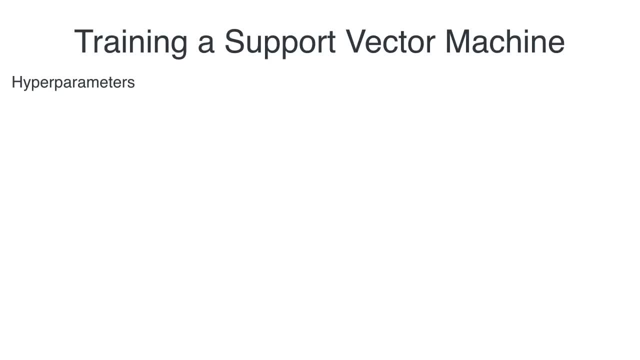 model is good. So what happens if we have more than one hyperparameter? right Here we only have one, which is depth. What if we're training a support vector machine? So in a support vector machine we have things like hyperparameters, like the kernel, which can be linear or polynomial. for 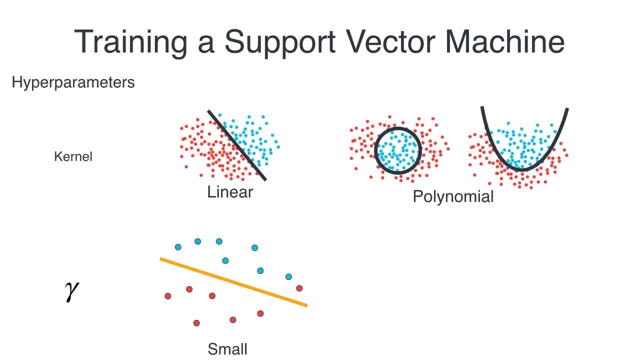 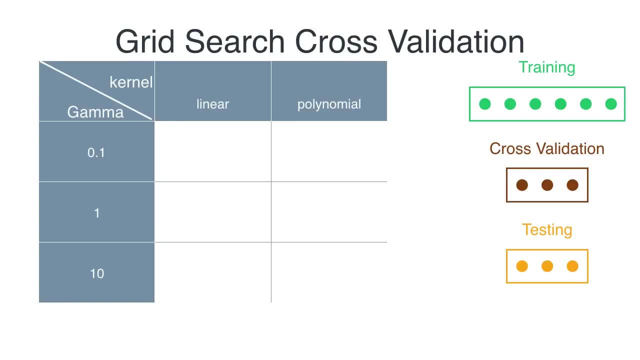 example. and we also have the gamma parameter, which, if it's small, we get solutions like this, and if it's large, we get solutions like that. And so how do we pick the right combination between kernel and gamma? Well, that's called grid search. We literally just make a table with our columns. 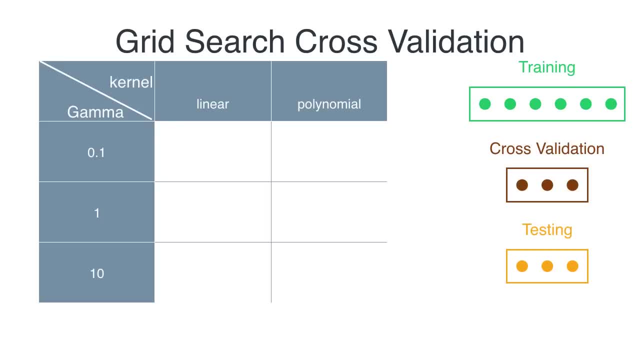 are linear and polynomial kernel and our rows are different values of the gamma parameter. So we take, for example, 0.1, 1 and 10.. It's normally good to pick some values that kind of increase exponentially, just to kind of swipe the whole set of values. 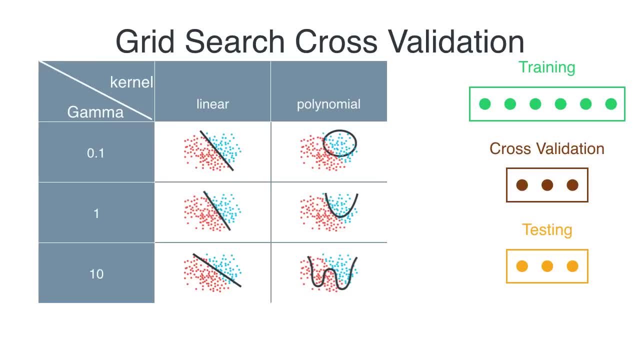 So again, we use our training set to train a bunch of linear models, a bunch of polynomial models with different values of gamma. Then we use the cross validation set to calculate the F1 score on all of them, and then we simply pick the one with the highest F1 score and finally we 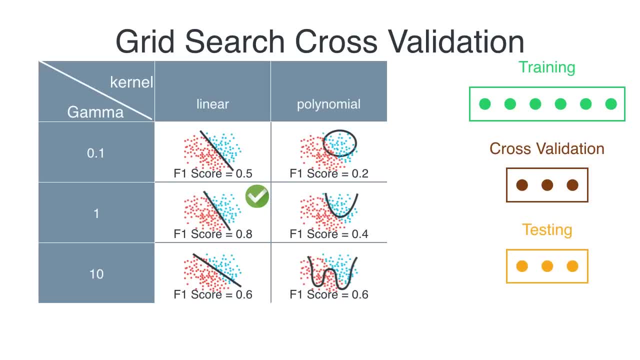 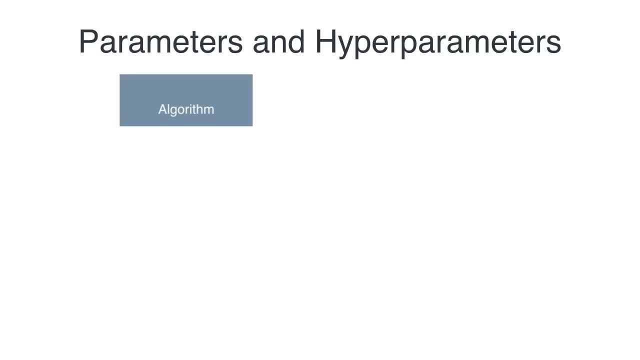 use the testing set to make sure that what we did was good. So, in summary, we have parameters and hyperparameters For certain algorithms. I'm going to tell you what the parameters are and what the hyperparameters are. So, if we have random forest, our parameters are things like: 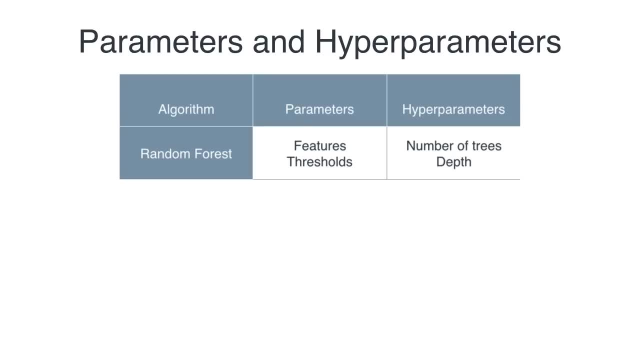 features, thresholds on the trees, etc. Hyperparameters are, for example, the number of trees or the depth For things like logistic and polynomial regression. parameters are coefficients of the polynomial and the hyperparameters are things like degree of the polynomial. For support vector machines, parameters are coefficients and hyperparameters are things. 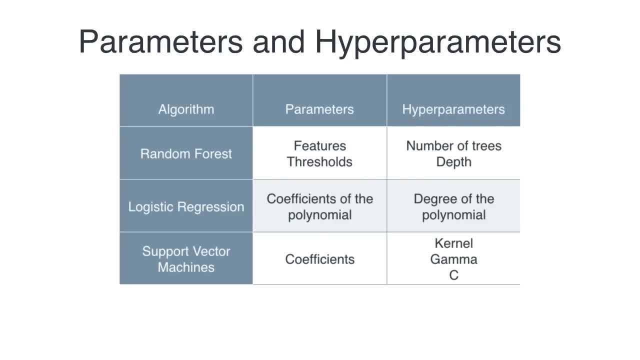 like kernel, the gamma parameter, the c parameter, etc. And for things like neural networks, our parameters are also the coefficients in our neural network and our hyperparameters would be things like number of layers, things like the size of layers, things like the activation function, etc. 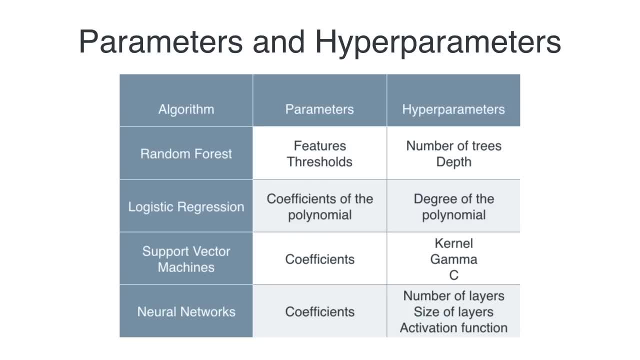 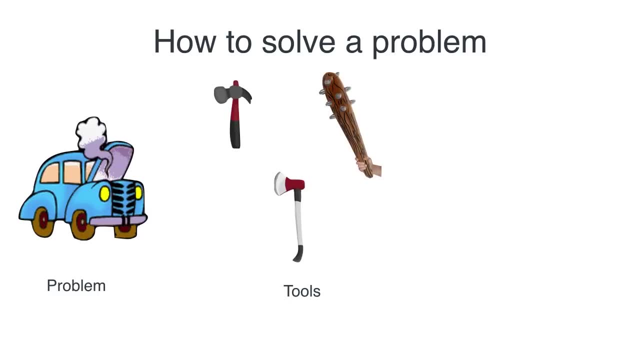 So, just to summarize, this is how I see machine learning. You have a problem that's fixing your car, then you have a bunch of tools that could be helpful for fixing your car or not, and then you have a bunch of measurement tools- which is what we learned today- and you use this.